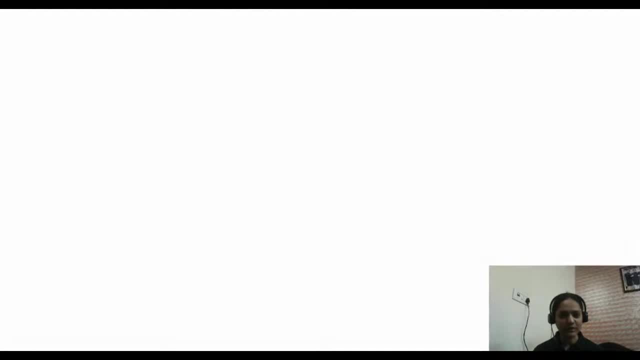 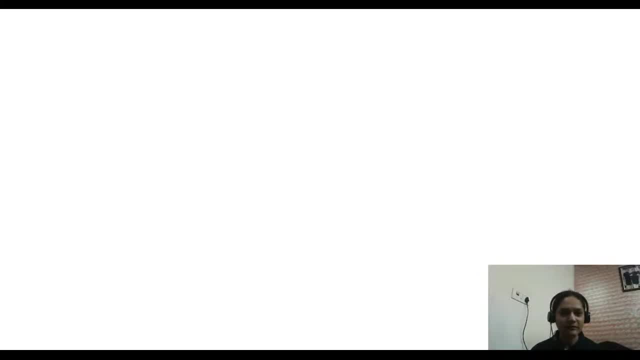 and also we are live on youtube and, as you can see, we had so much fun learning uh about python, upskilling uh ourselves, uh, during all the life that we had. and if you want to share your opinion or anything with us, do give us a shout out. on social media also, you can connect with us. our 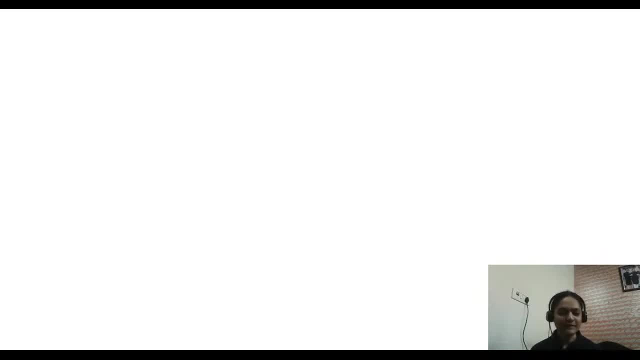 team. we are always happy to uh, learn from learners and also, you know, work on a work based upon the feedback right? so, yeah, looking forward to seeing more learners killing themselves. you know, make joining this data revolution and, as you can see, we have. this is one of our last live class. 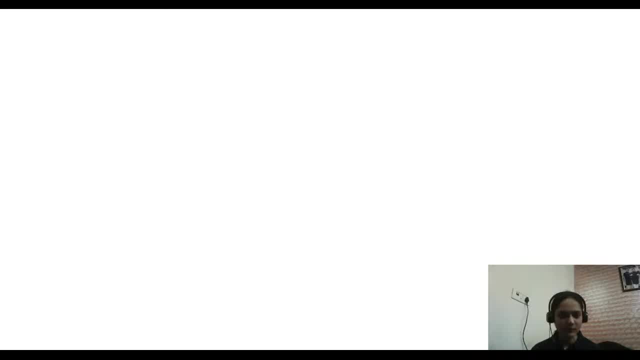 we covered uh from basic and escape and today we are going to be covering the final python case study. so just before we start our case study, let me just clearly recap during this session: uh, if you have doubt- and there is- please feel free to pop it in the live chat. 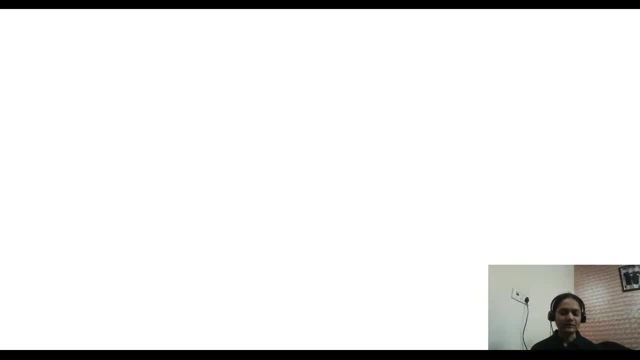 i look at it from time to time and and i will answer it to you directly over the during the session of somebody from our team. answer you definitely in the chat itself. right? so how we started around one month, or have we started with the basic of python like python, python uh? 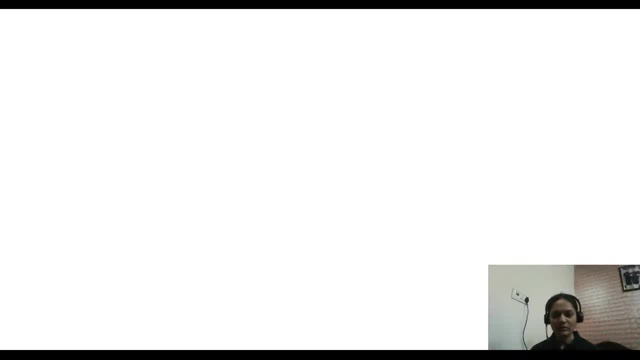 language, basic fundamentals. also. we started we covered some data structures, data structures of python. then we covered the different functions related to those data. like you can say, list hair strings have all the important functions related to need of structures. okay, bad weeks covered loops and funds in any Python. 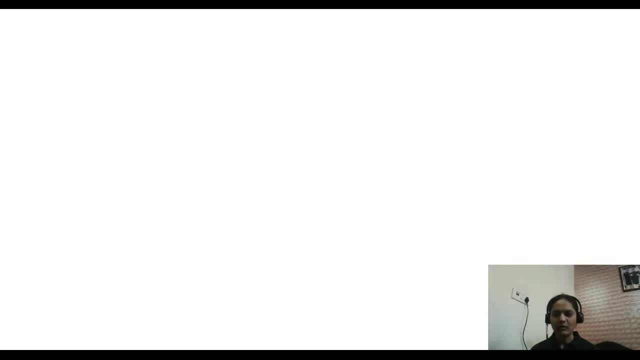 program, which key, how do we create a loops, how it up function of Python, may modules they like these packages and after that we move to the exception hand like a pure code. my coi error at the to say related on exception in error handling him. can circuit accord may ordinate about become the concepts of 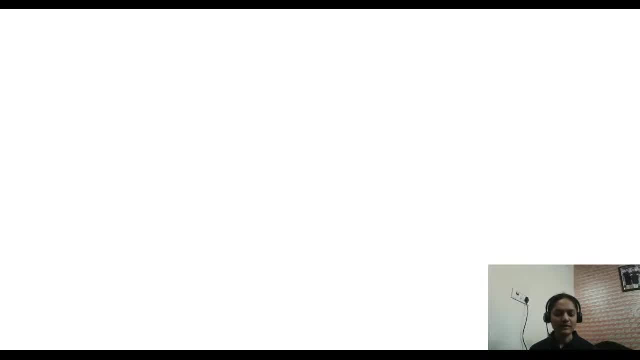 who and classes casacreator they have and what different types of oops in oops concept? or was Caucasus pm cast? if work could they have are create a real world scenario project. project containing: and right and as far we covered, different data libraries. Joe Python, may that are like very cool. 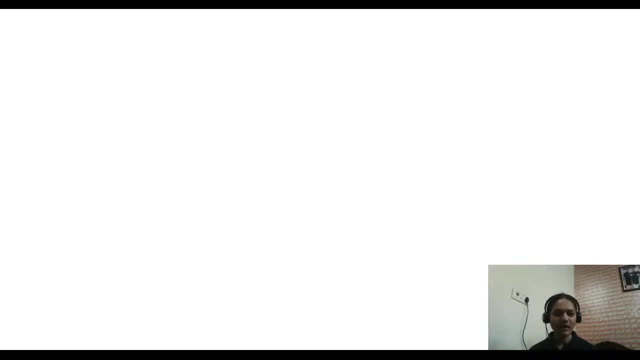 different data libraries to Python may that are like very cool and we covered in which we cover three most popular libraries that are pandas, numpy and matplotlib. now summarize all this: today, using all that we learned till now, we will do one case study of python case study, as we have taken a real world scenario. 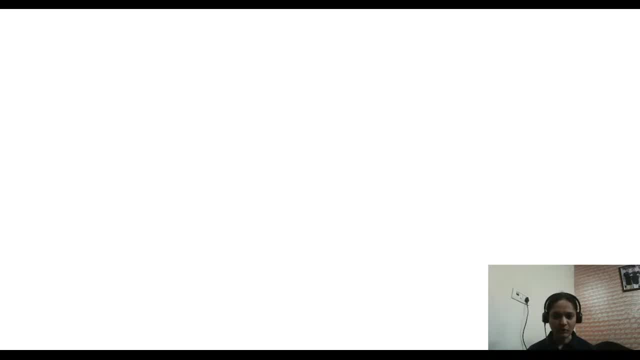 and we got some data about product and on that product we are going to be exploring that data and on that analysis, how we can make it useful for teams or for our company or for different use cases. so just to the scenario, and before that i'll have a quick look at the live chat. 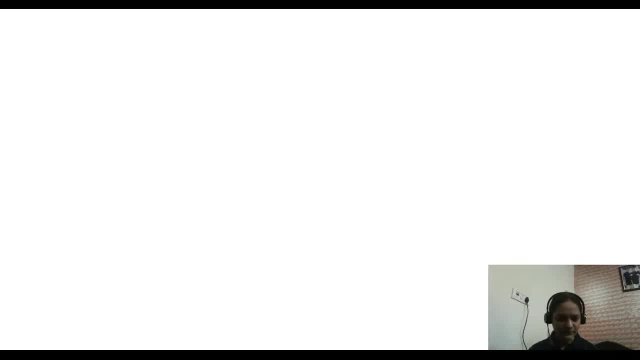 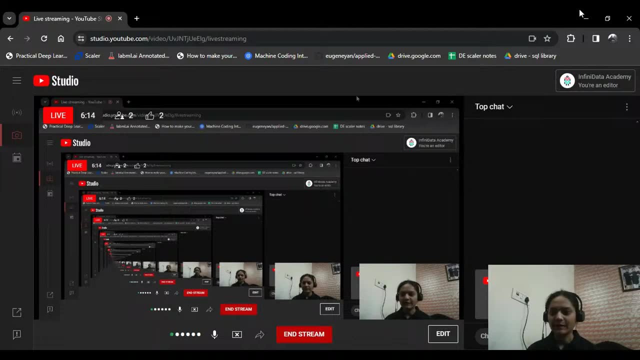 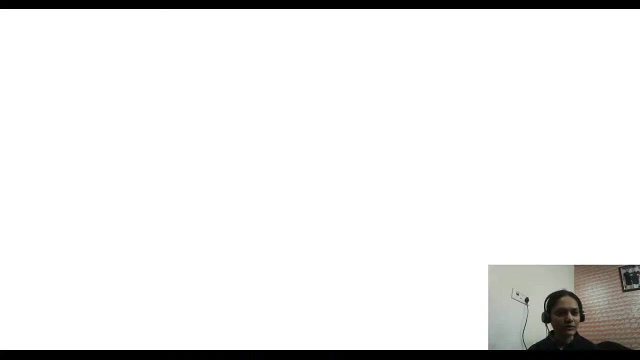 and see if anyone has any questions. please feel free to all right. all right, all good at the live chat, and so i'll just start over here. so this is this time i'm using visual studio to show you this code study. so i used visual studio because it is one of the most widely popular. 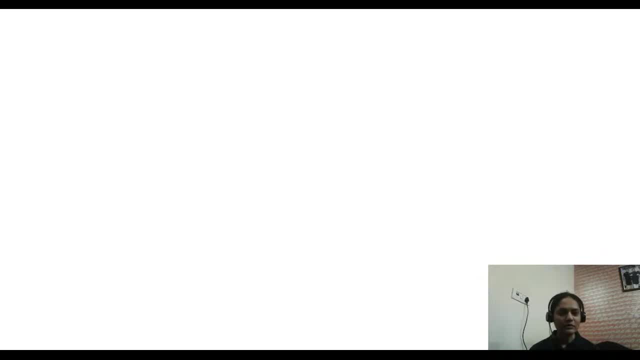 uh, ie out there for python and also there is one use like visual studio is also very useful in this. we are using jupyter notebook like we were using google code till now as a notebook. the same way, we can also use visual studio like we can execute our code. 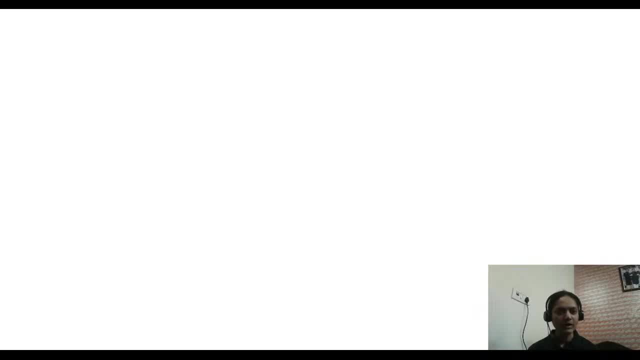 in a in the same way, in the format of a jupyter notebook, directly in the IDE itself. right, so over here, let me just start. so, first of all, we imported our libraries. and what are the libraries? we discussed different libraries, which we have done so far: python, pandas, matplotlib. 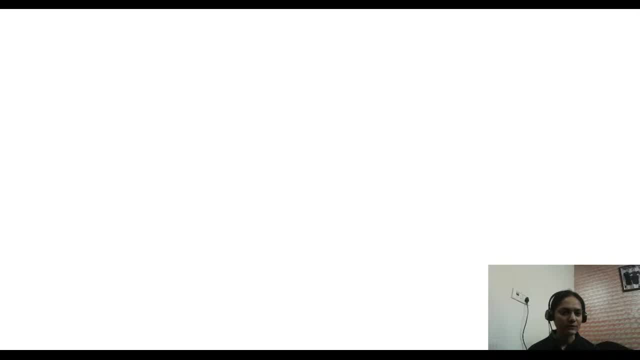 then there is os, then this re is for regs and we have beautiful soup tqt. all these libraries are there and basically these libraries we will use in today's study to uh. to conclude, a conclusion. so we are on case study. so for today's case study we have scraped the data for popular product that is, iphone 15, which is the latest iphone and series of iphone models. so in that iphone 15 reviews we have scraped from a popular e-commerce website and from there we have scraped, we have set it in our local system, like my local. 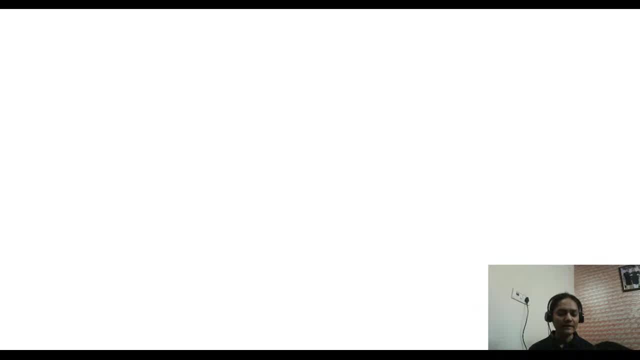 system as a csv file and then, after reading that csv, i have just prepared this notebook, what all we can do. so this please keep in mind: case study is, from a point of view, from very basic, because we have covered basic sessions. if you want to do some sort of advanced analysis, 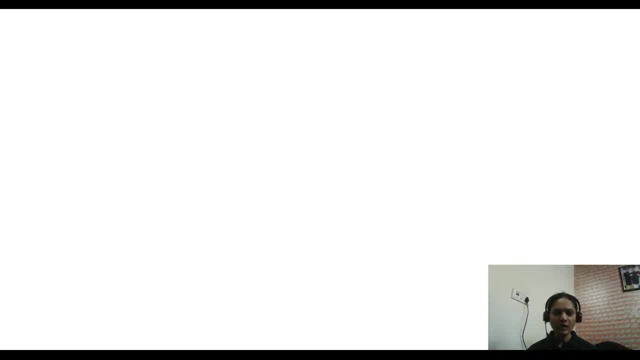 over this, then obviously you can, you know, go for, you can contact us for data science courses in which we will be doing more real advanced cases, but this is from the point of view of the beginner learner, right. so let me just start with this, and so, first of all, 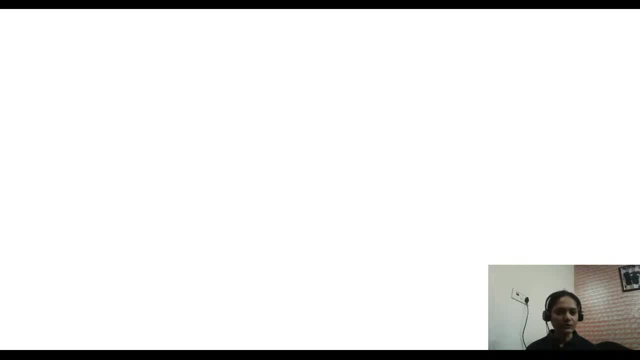 we imported our, we are using so for, like, we have pandas for data, data visualization and also there is a library. that is basically so status you can use, and then there is a- so this is for the natural language processing, so you can use this kind of you can use. 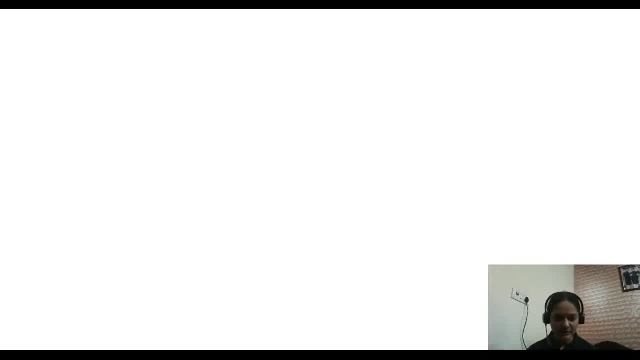 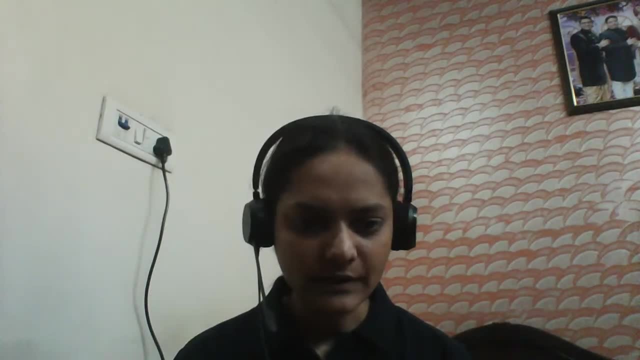 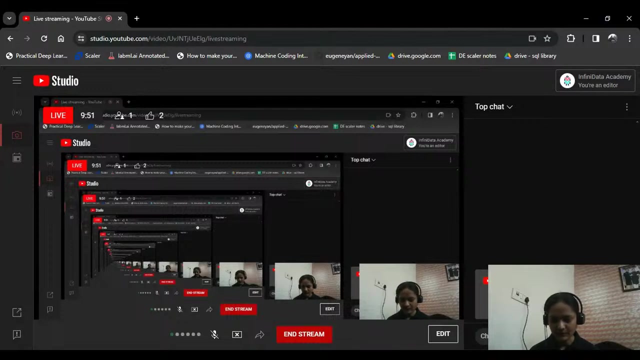 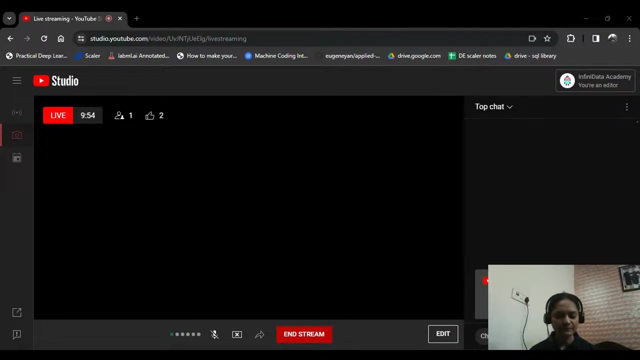 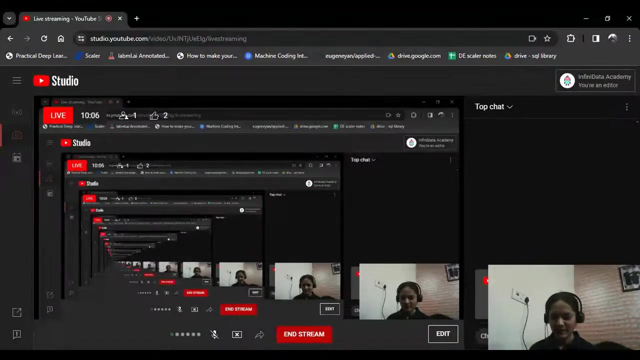 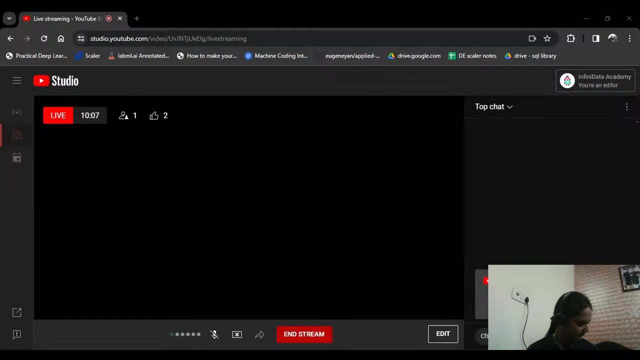 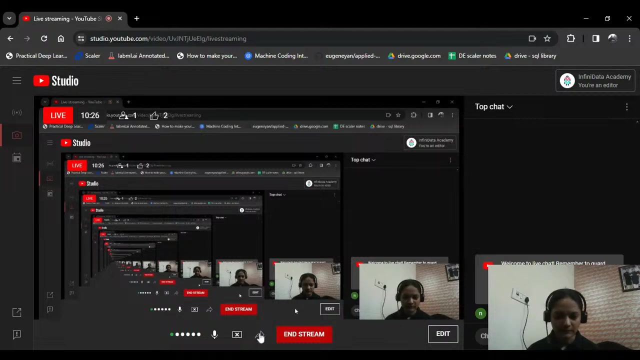 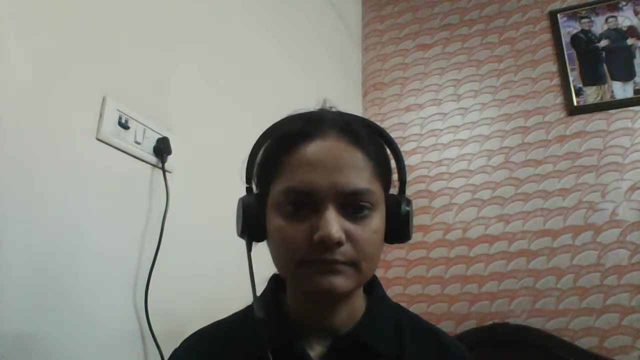 this to. you can use this to. you can use this to to to. okay, can somebody in the chat tell me if my screen is visible or if you can see that this visual studio code vs code screen? okay, you can just type yes or no. black screen for a on camera is visible. okay, I will share again. okay, I hope it. 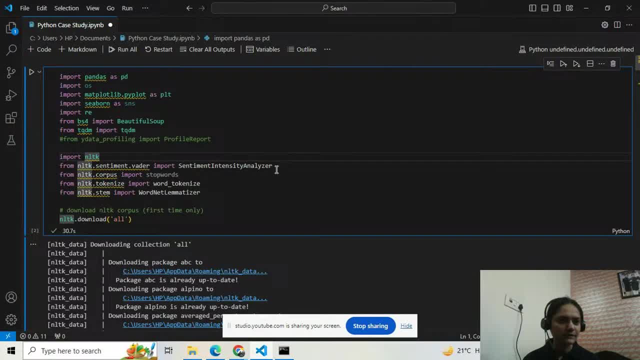 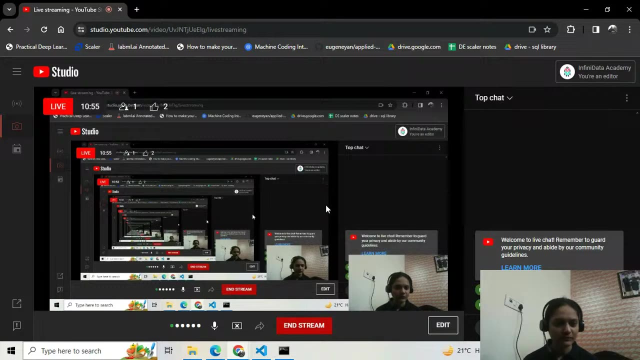 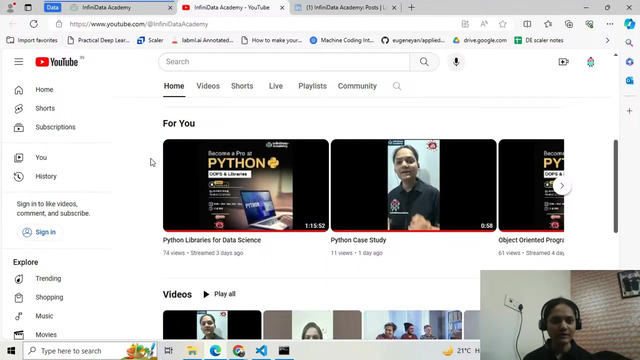 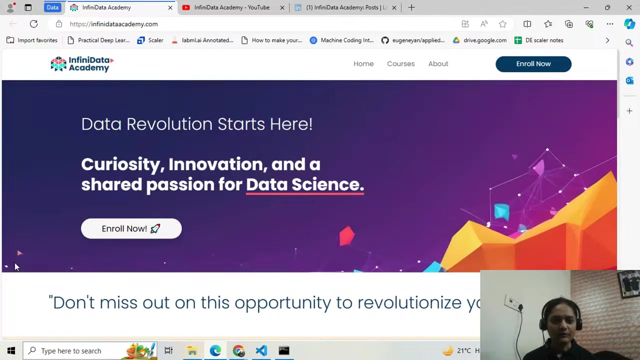 should be visible now. is this visible, the black screen that I have here? okay, thank you, Nia, for confirmation. okay, all right. sorry guys, I think whatever we talked longer, your context could be mixed with what we said. just to reiterate: this is our uh website. that is infinite academy. just say: we have uh, we put on our 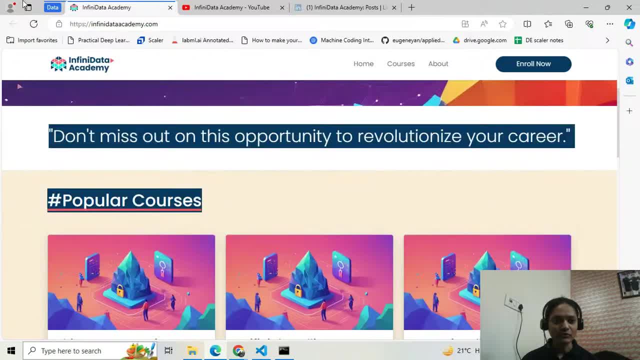 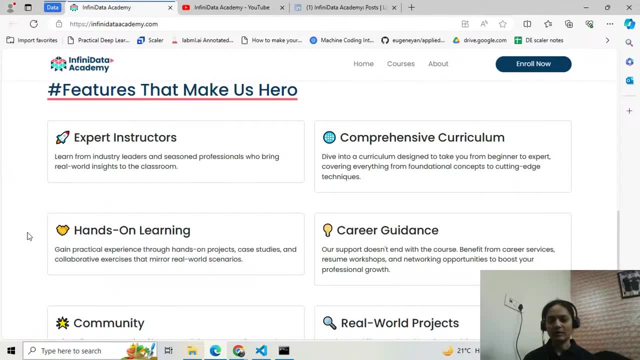 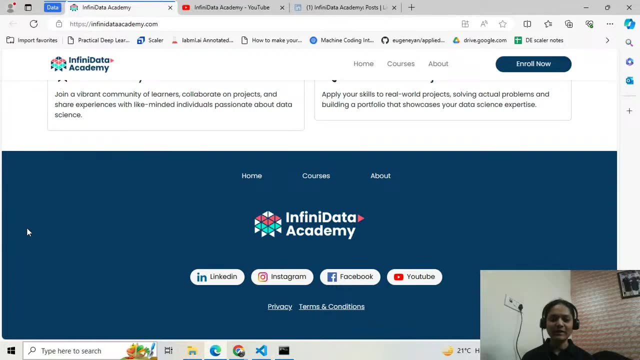 data science course. they're going to be launched soon. and also you can get in contact with our team for any uh career or you know to, about our uh sales, what is our uh? and also you can uh follow us on various uh social media channel linkedin youtube. we are at all of these channels and, as 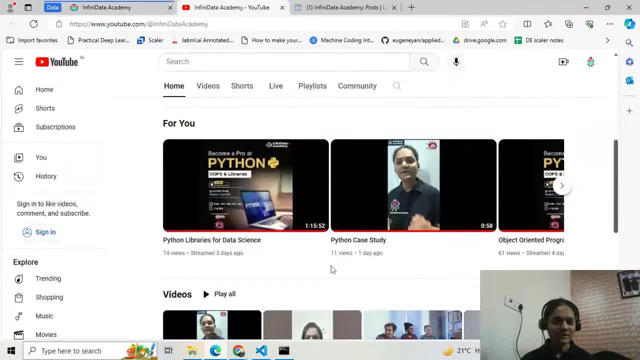 you can see our youtube channel. abhi, this is the our last class series of python classes which we have uploaded. we have uh python classes for the last one month over the weekends and i hope you guys have done the session and also have this uh infinite data. 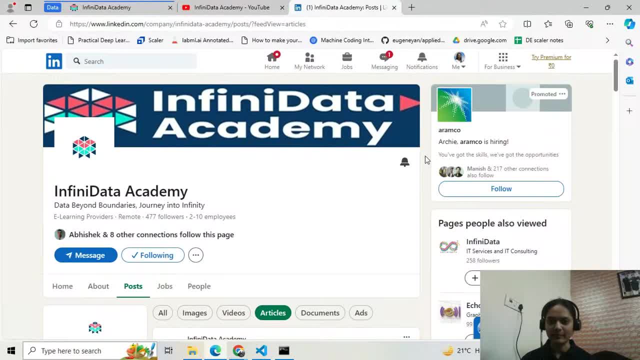 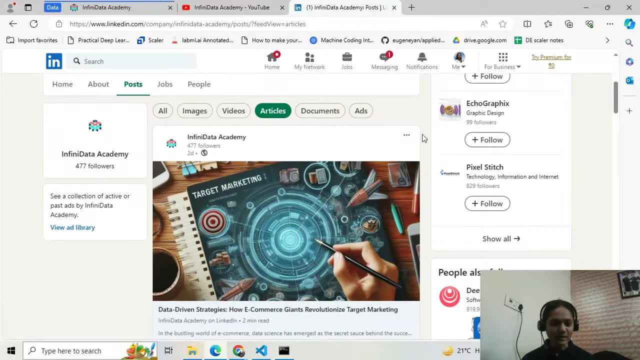 in channel or linkedin page over here you can see we are putting in different technological articles. we uh discuss about the waste industry trends or emotions that are taking in the field of data science. so keep in uh, keep in touch with uh us. please do for this uh page and, as you were saying, 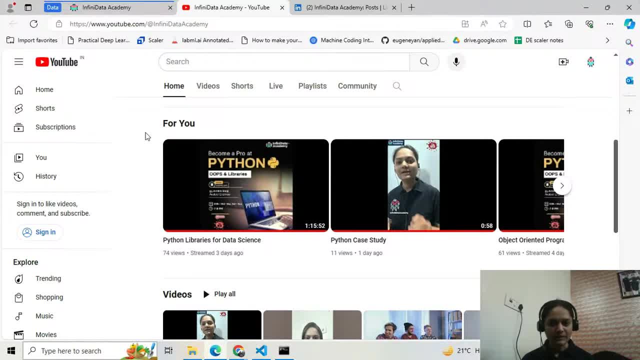 we started from very basic uh from python and data type data structures in python. uh cover loops, functions and functions and also how to create classes in python classes. and finally, in our last class we discussed the different data science libraries, three most data science libraries that are most popular in python, so that the pandas, numpy and matplotlib- so what you know library. 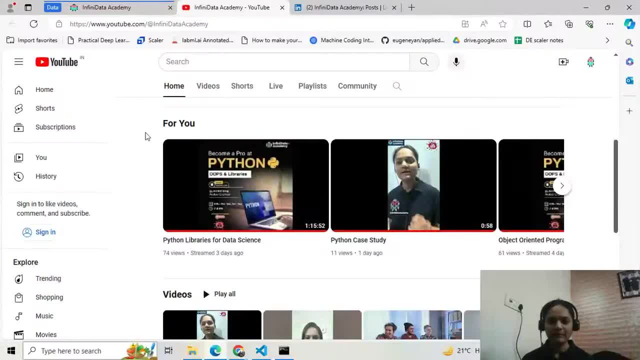 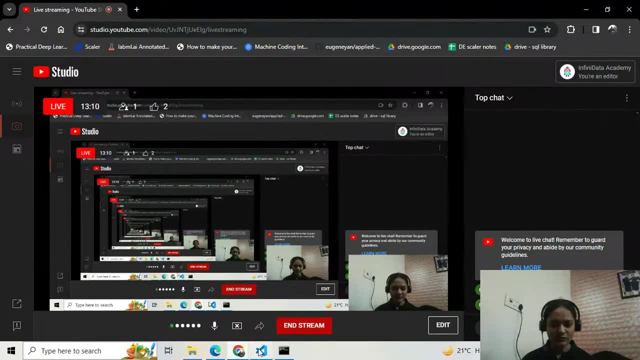 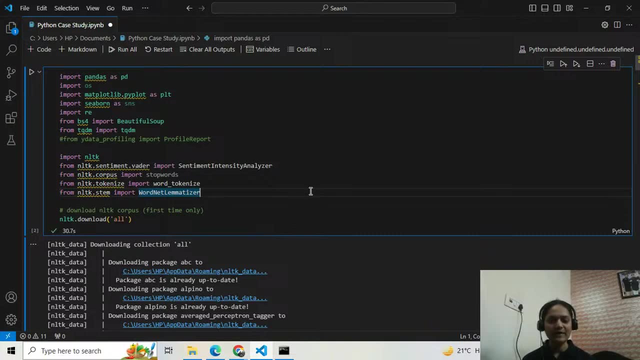 also, uh, how, uh, how, we can manipulate data, vision data, using those libraries. so which uh brings us to our today's case study. so today's case d is a sentiment analysis: these reviews of iphone 15. uh product from a popular website and put it into our local stem as a cp file. and 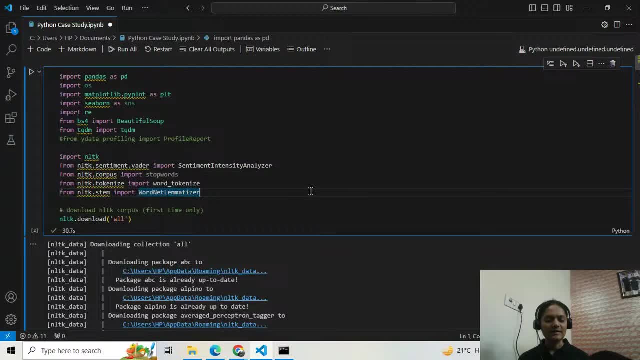 we are going to analyze this data and see, uh, what people are saying, update like, if people are more positive about the product or negative about the product, and also what takeaways we can get from that, from those reviews. so before we start it, please keep in mind: yeah, this is very uh basic case study. there are more. 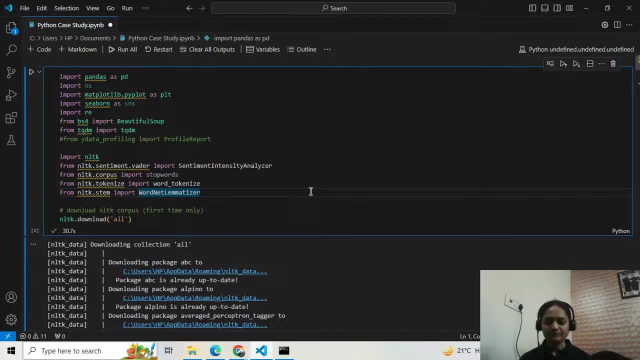 advanced vacation and also modeling that we can. on top of this, and to know uh more about how you can operate data science to your current scenarios, current project, please do get in touch with our team and we always look forward to uh connecting with more people. right, so subset family. this is a 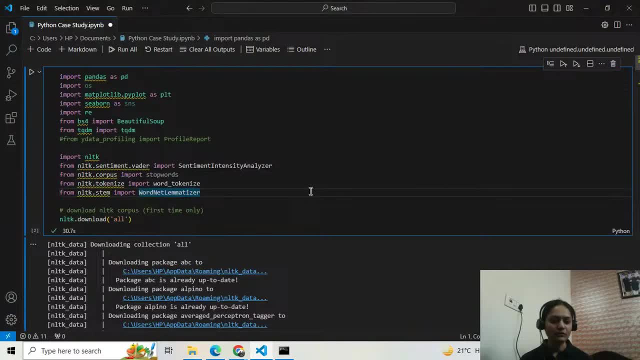 and then for the data sheet. we have uh. we have a lot of uh. sellers have a eyebrow habit because of the fact that the app does not outline data from the login, but it is fine, so we will go through each and every one, based on the data of. 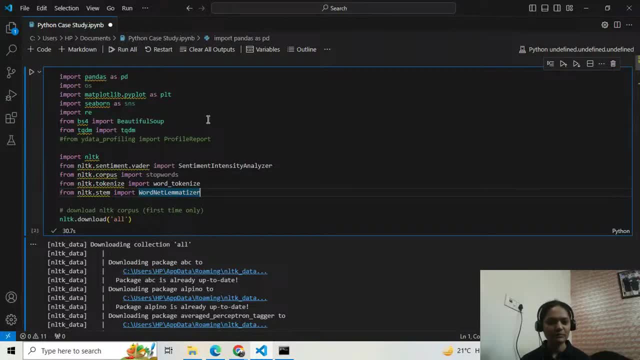 data and uh, for that use case. awhile data و explain now. okay, today i am going to tell you how do i pull out the data and see the pressure process once again. let me talk about the data later on to test you what we should know, and also we should also know what quality is and after seeing this data, since before writing data, this time we need to learn a lot of data. so that's why i am giving you gl374 if you can see this data, if you want to know more data, test. so this letter is adj. 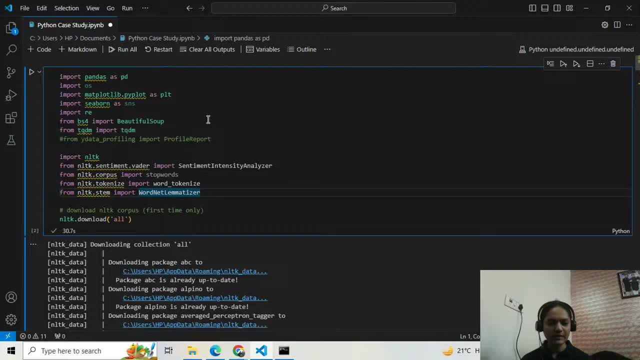 uh, we will see each of this. just a code code go through. we will see how each of are used. then we have the nltk. so nltk is a natural processing library so up. so this is a very popular library for nlp. uh task so up different, different language may job. 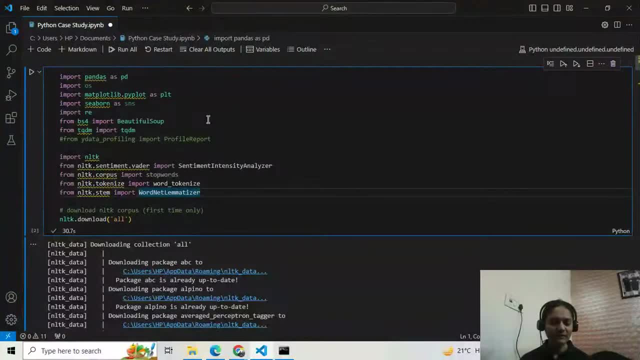 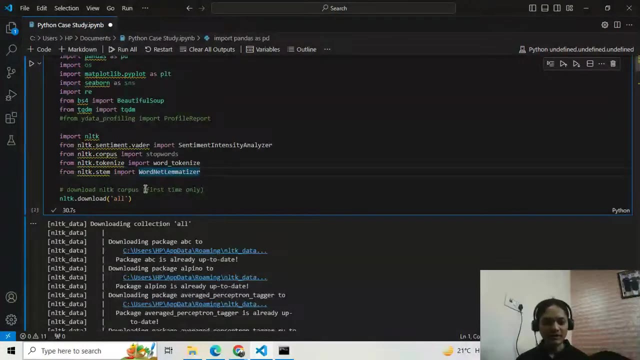 like sentences. so this library is very highly effective and useful. it has many pre-built uh functions for us to use directly as it is after doing pip, install ldk please, uh, nltk, dot download in your system. so this download all basically different languages. like you have so many languages- english, or you know. 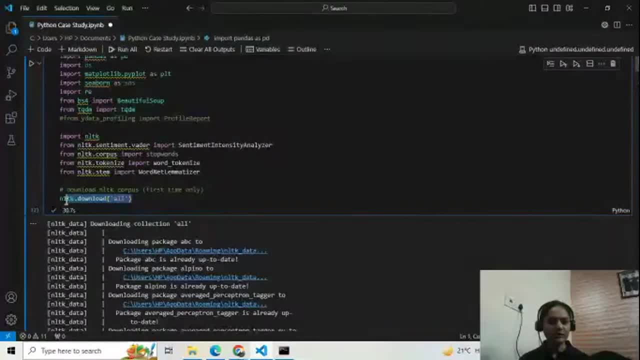 all those packages, local, stem, and so you don't have to, you know, uh, re-download it uh every time. uh, so this is going to be only one time thing, but it's going to take a big fight, right? so, since all these packages installed, so that it did not take much time, 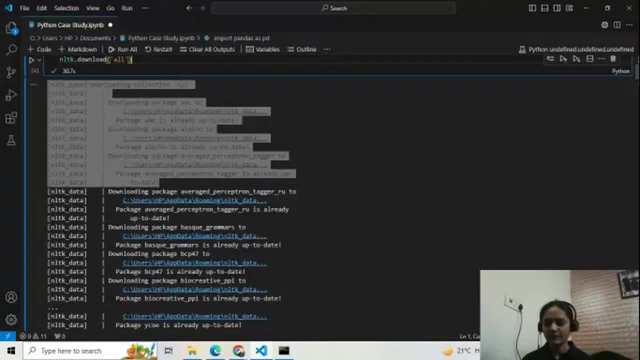 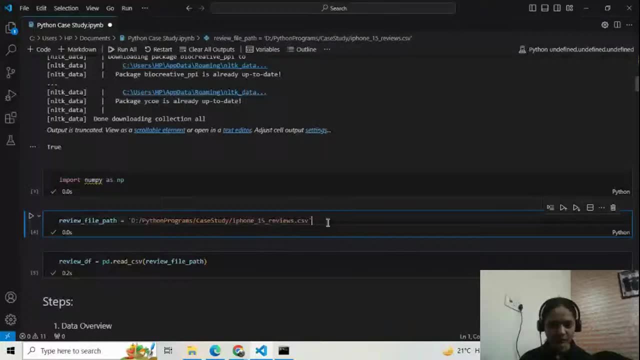 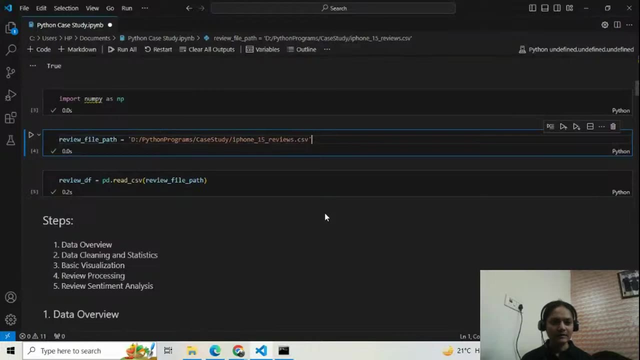 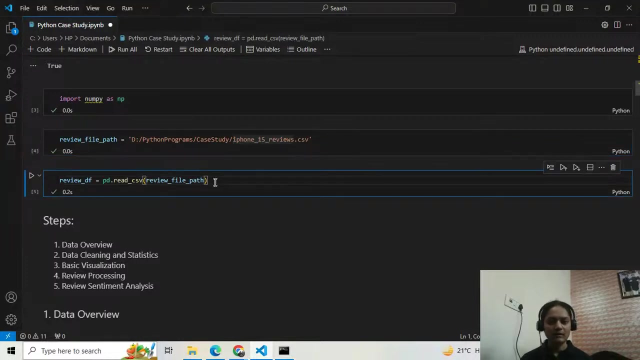 oh, let me just a click in and it worked. apple, uh, this is the thank god. after that, you will love it, we will see. okay, so here, uh, so abhi tak humne. we just imported the required libraries. now we'll start the code. key code of the machine. dca. and firstly, this is basic, like i have taken the reveal path, or what ah the file? my name of the file that is iphone 15 review. so jours he this csv file just may have missed data. uh, loved kia rez. open the current system. 5ment in dsk. need grew in this sugar system. 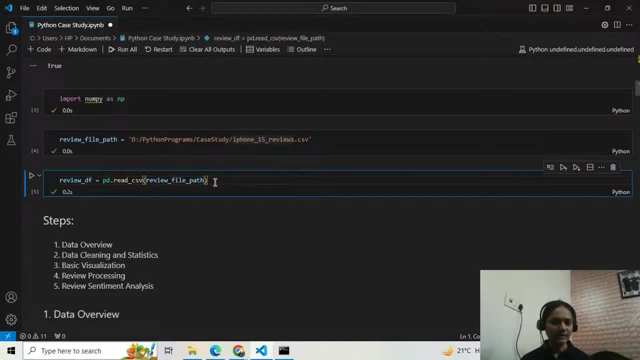 48 Garicore sensor. he know where the phone and Skype application is fixed. interested in getting the screen code as well? then you can please give us a message on LinkedIn as well and we will be happy to connect with you to tell you more about how we scrape this. 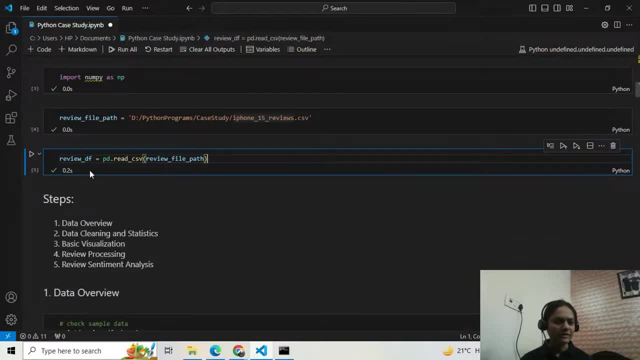 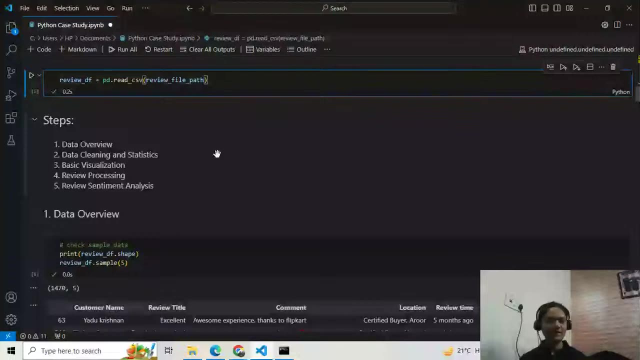 data and so I am just using pandas. so pandas alias pd. I am just reading the csv file and I am going to discuss what steps we have taken on this. so different steps which we have covered. that is firstly, simple, brief overview and then the six steps over it about the data and how to 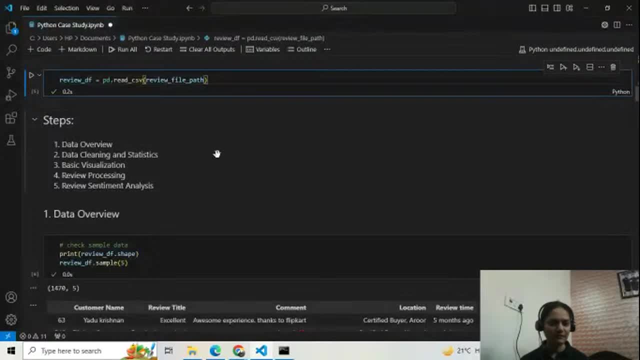 clean this data and do some visualization that we have done. after that we have to process the reviews because we cannot use those reviews as it is whatever we have scraped. we need to process these reviews before we can do the sentiment analysis and then, after assessing, we finally 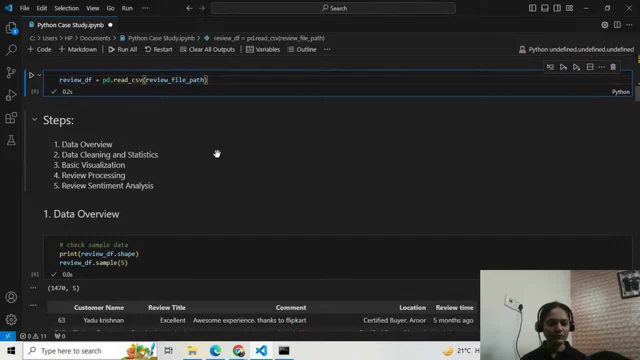 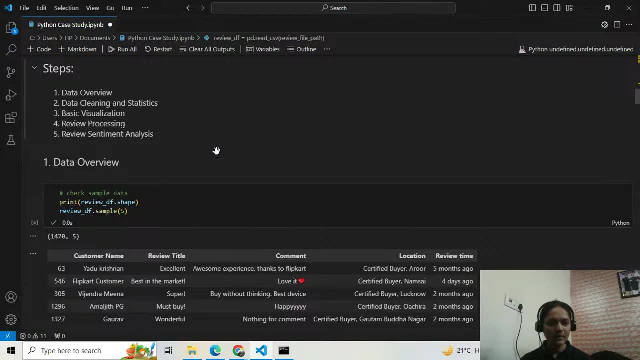 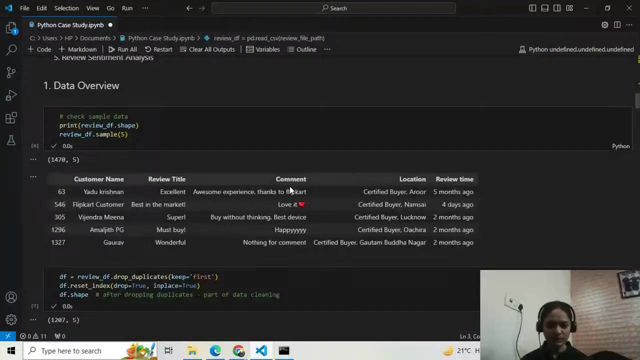 do the review or sentiment analysis of that of those reviews right. so start with the data overview part. start just to reiterate that if you have any question or doubt, please free to put it in the live chat. I will keep on going to the looking at the live chat from time to time. 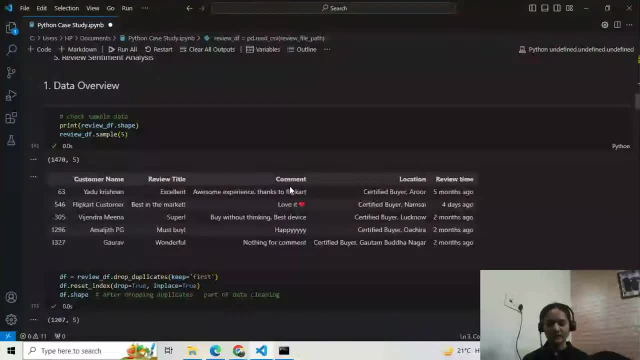 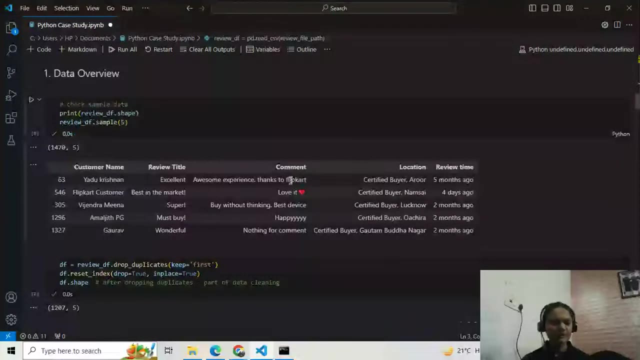 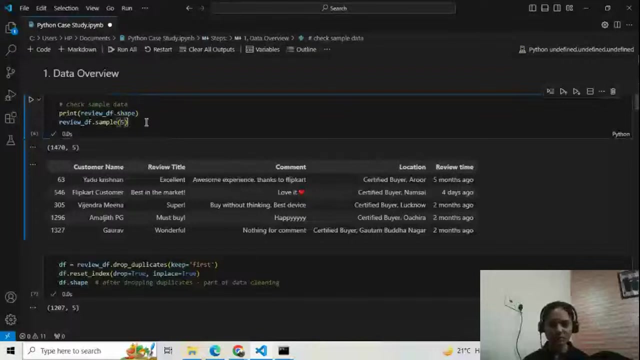 in between and we'll see that, whatever your question is like, side by side, it gets answered and you do not have to wait till the last for it, right? so let's start overview. so first for all that we have scripted, we are just saying that how many number of rows are there? and just a small. 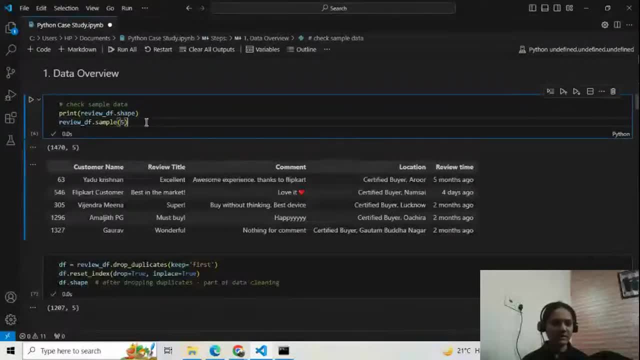 sample step data. so you can see, in our we have five columns. that is customer name and then we have the review title and the comment location and the review time. all right, so in this you can see these emojis, emojis and, uh, some you know weird characters present at times. so 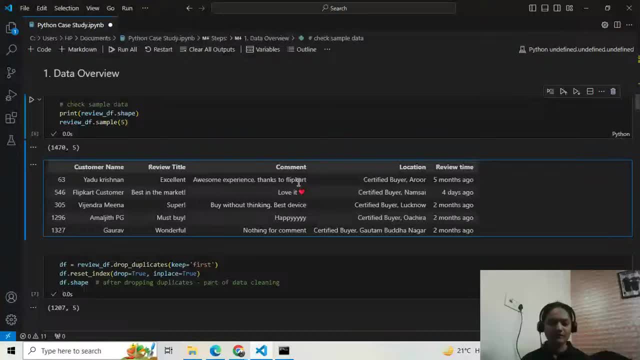 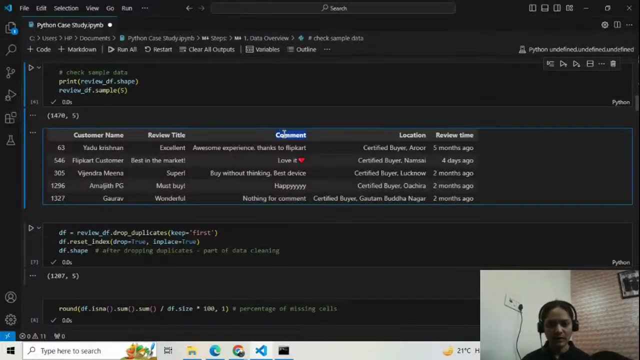 basically we will using comment, this we will be using to analyze also. you can also use a review title as well. so at the end of it end of the today's, if you are interested to know or to use the review title as well so you can take it as a work, then your title, you do the sentiment analysis or, you know, combine. 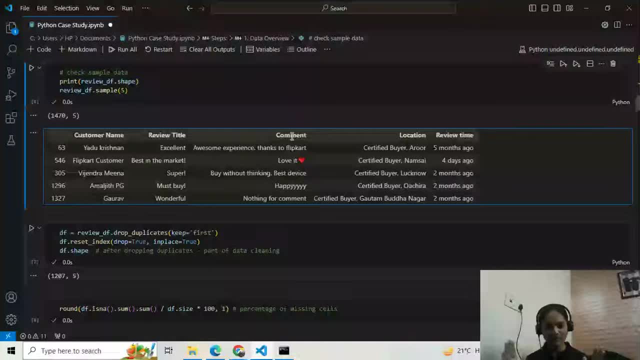 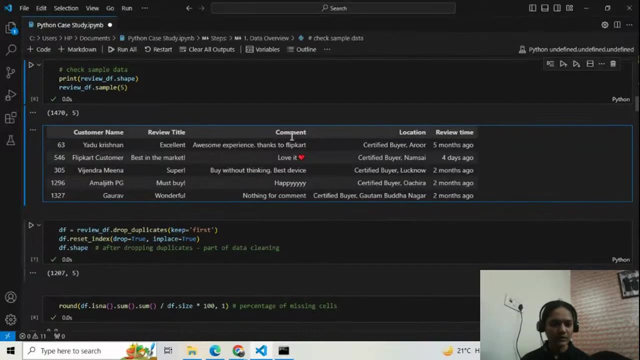 review, title and comment and then sentiment analysis over it. so yeah, so yeah. but uh, for today's case study we have the comments to uh and to get sentiments of that review right. so so, in end of this, uh, first, the first processing we have done, that is, dropping the duplicates. 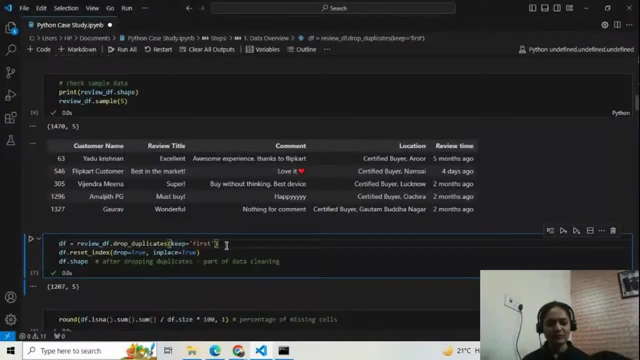 so in uh, in any data injured, many times duplicate values is present. so that is uh, there are multiple of it. human error or maybe the code error, the duplicate will get added into our data. so to drop duplicate pandas there is a drop duplicate function which i have just. provided this parameter, that is, keep first. like if you have got 2-3 multiple duplicate pairs rows in that, keep the first row in your final also, since also in duplicates you can define how many columns you have to duplicate, let's say where both are same. 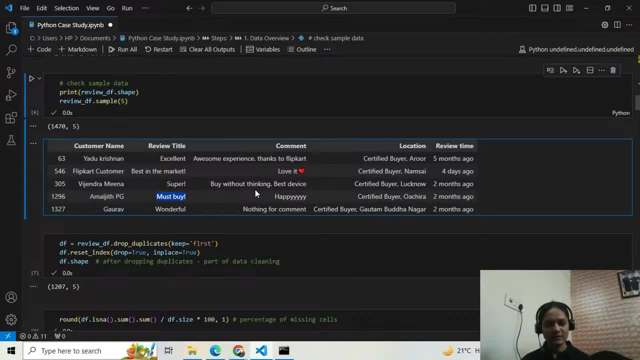 both are same, like if in this row, in the row 3 and in row 4. in both rows if review title is coming, then I have to drop one row. I don't want to worry about customer name, location, review title, both can be different. 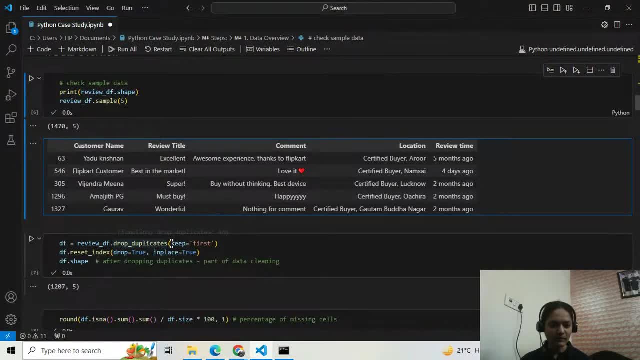 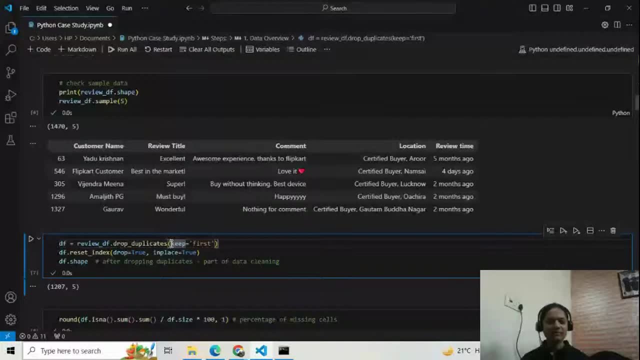 so it also provides a parameter which is subset. you can also provide subset. drop duplicates only on the basis of 2 columns. on its basis, then you can drop, but in this we are just containing all the columns. so that's why subset is not provided. so we are just containing all the columns. so this is basically reset index. whenever we drop the index which we have dropped default reset, it stays the same as the original one. to reset it, you can run reset index and then drop true in place, equal to true. what is in place equal to true, it will make change the data set. in the data frame itself. like you don't have to assign it df equal to dfreset, you don't have to do index. it will make change in the data frame directly because of in place and after dropping duplicate, we are checking the shape of the data frame. 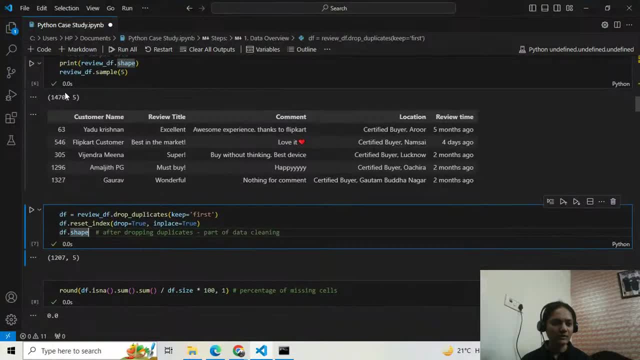 now like how many rows are available. you can see, out of 470, we have 1207 reviews now. so this tells you that in the data we have 1270 reviews now. so this tells you that in the data we have 120 reviews now. so this tells you that in the data we have 1270 reviews now. 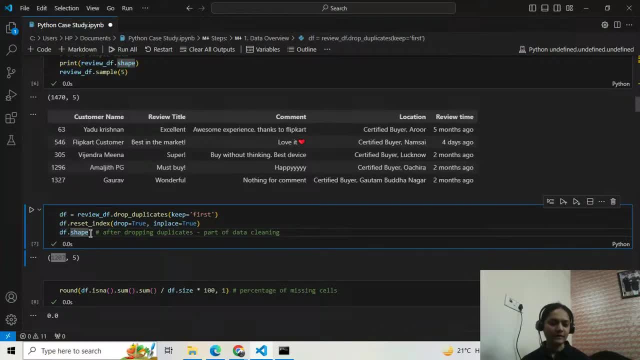 in the data we have 260 reviews. the reviews were duplicate, so basically we don't need the duplicates because it will skew the final output. so that's why it is always better to do duplicates. and there is one more thing in the data that is the missing values. 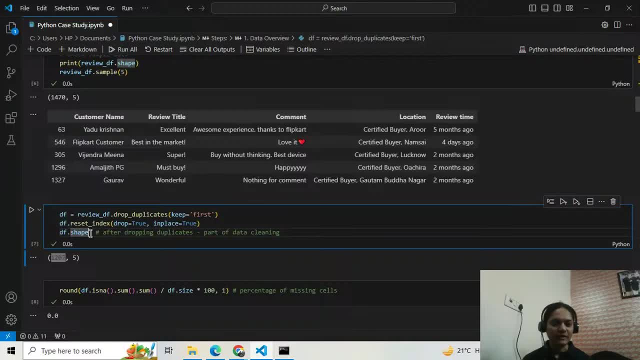 like in your case. let's say the name is missing or comment is missing, so you need to find how many missing values are there in your data and you can either replace that or you can replace that column or row, so there are multiple ways to treat those missing values. 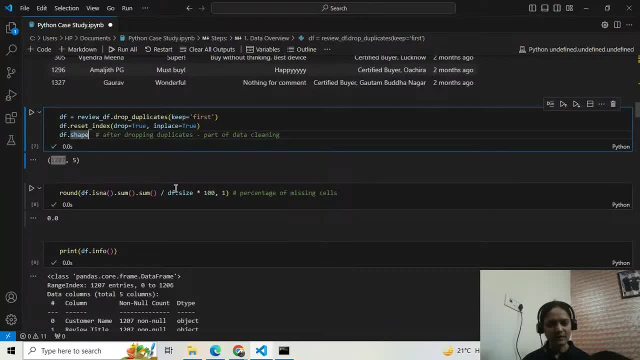 so in this case we are just checking that. are there any values in your data? this is just the formula we have run like data is a quadal value and then we are dividing by the size, which is an average calculation formula, and we can see the output. 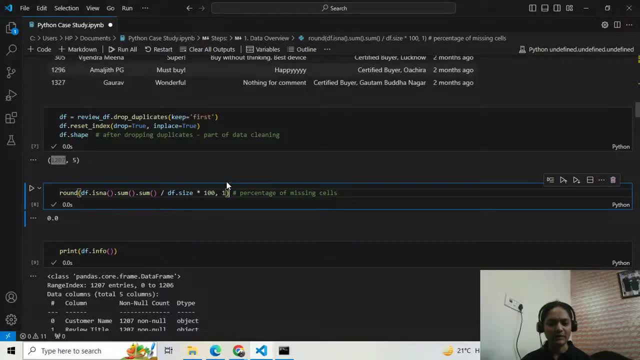 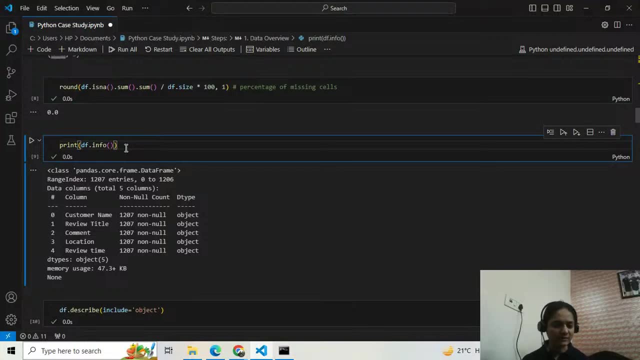 is 0, so there are no missing values in our data. so, as you can see, if we did dfinfo- dfinfo, we discussed in the last session- it provides information related to your data frame. so, as you can see in this column, it is showing 1207. 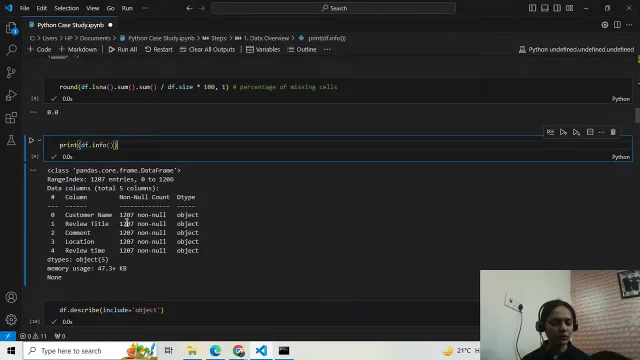 non-null values. so there is no missing value, there is no null in your data. so good thing here is that the type of your data in all columns is object, basically because it is showing text value and string value. so it is showing it as an object over here. 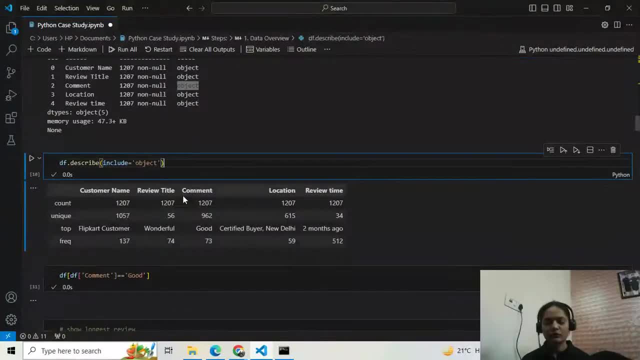 right and if we do a simple drive over it, so describe in numeric case. it shows you the different personal values and as well as standard deviation. but since here we only have- we only have string values or text values, so that's why we are just getting these four. 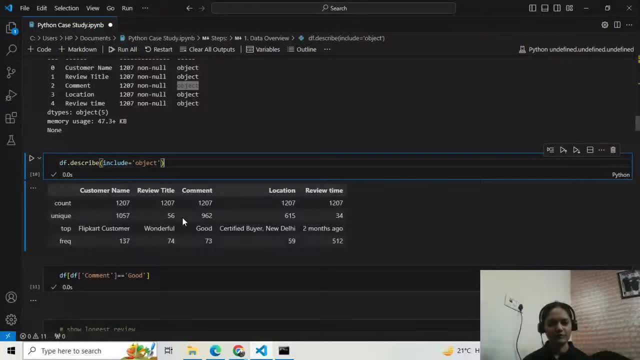 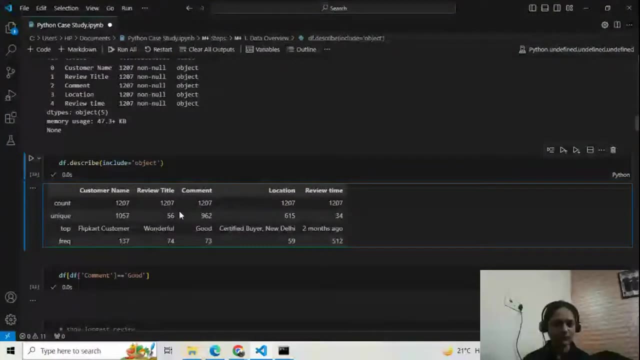 these four metrics like count. we all know count is 1207, but after that we can see its unique values like there is very less number of unique. there is lot of in our review title and same for our review time. so review time understand like within a month. 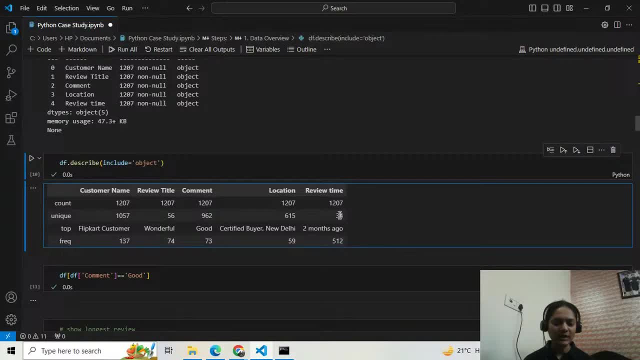 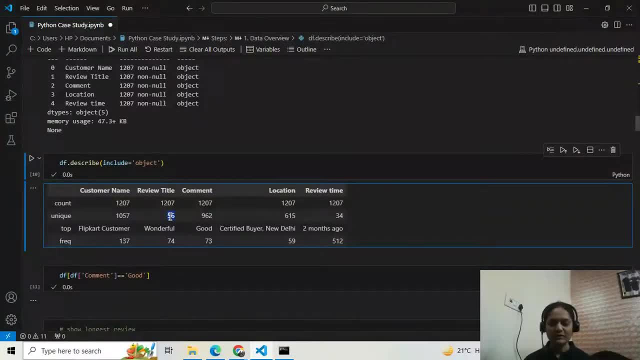 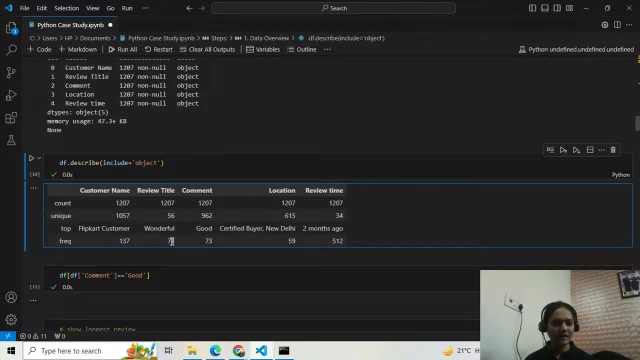 you can see 24 times joe b title: that is just one same with comment: media case may: uh, people just put good and that is around 73 times. and location: you can understand like there can be multiple people reviewing. so you can see the new delhi is the location in which 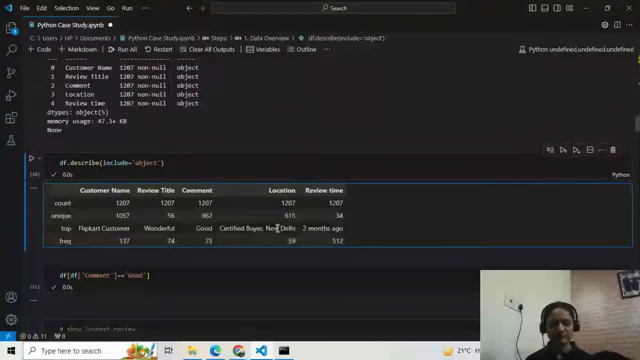 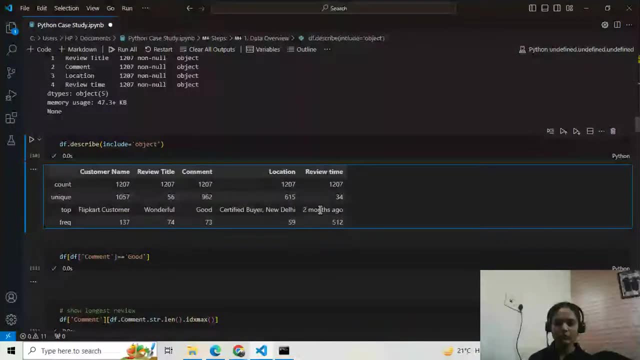 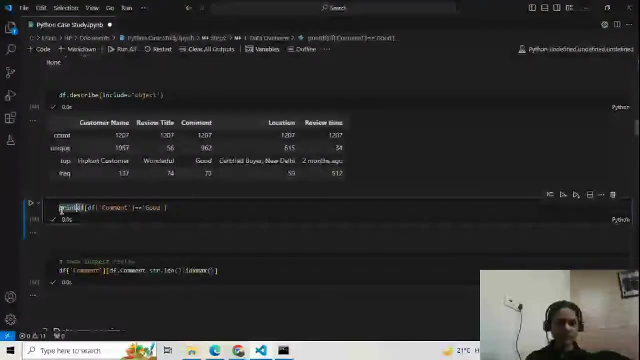 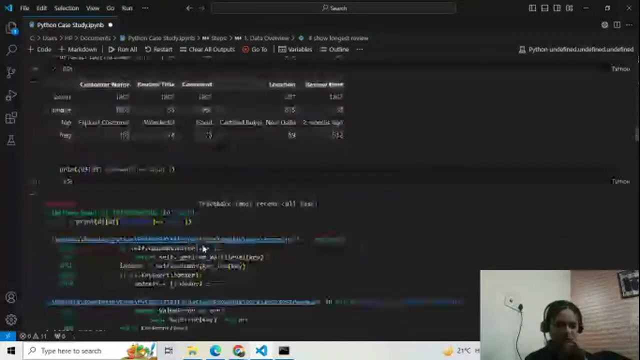 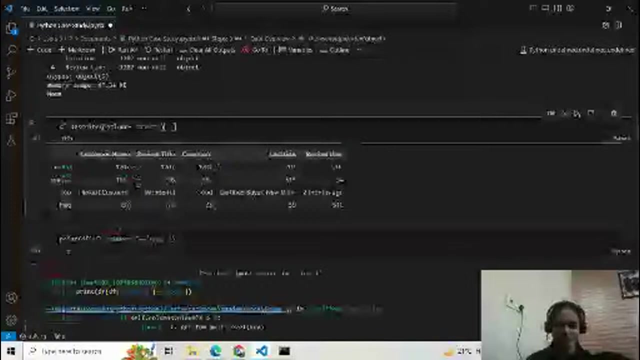 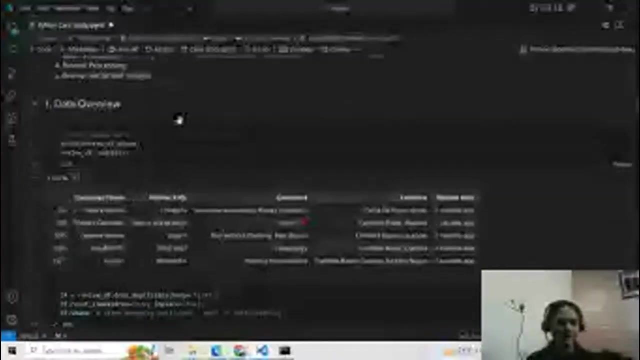 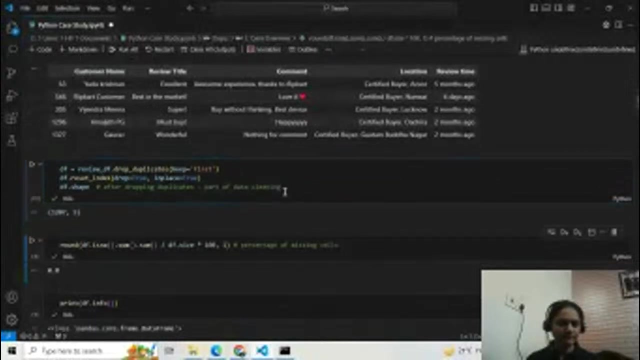 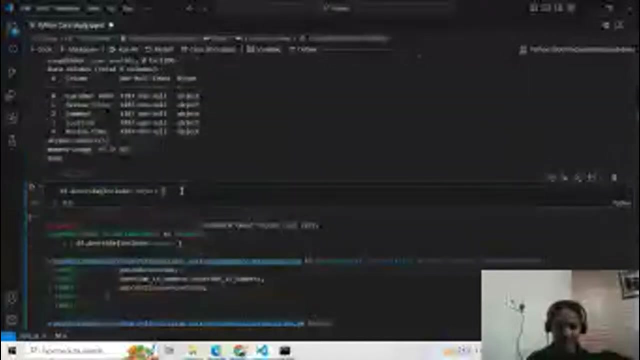 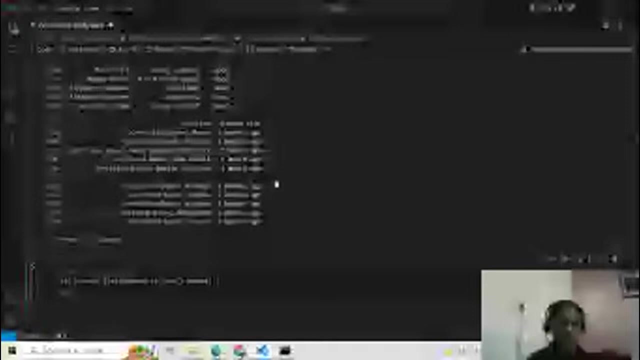 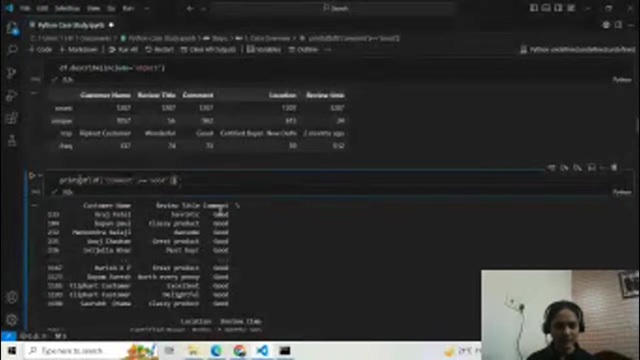 highest number of people have reviewed uh, the iphone 15. right same way, you can see the review. uh reviews joe scream. always the is good. yeah, i think it's go rerun. let me just rerun nature. we have done some manipulations already. um uh, okay, so you can see now like different types of reviews. mess, if uh comment is just good as you. 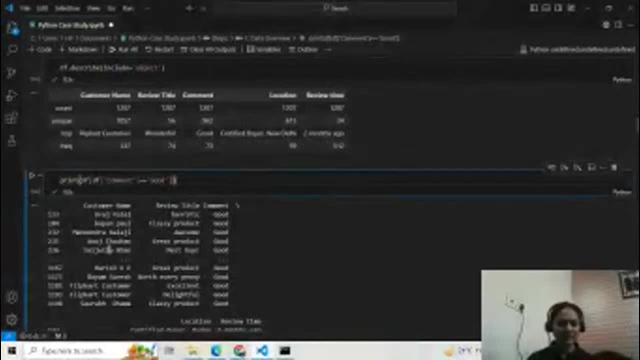 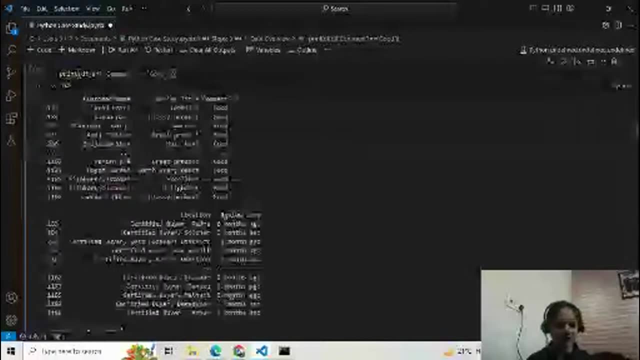 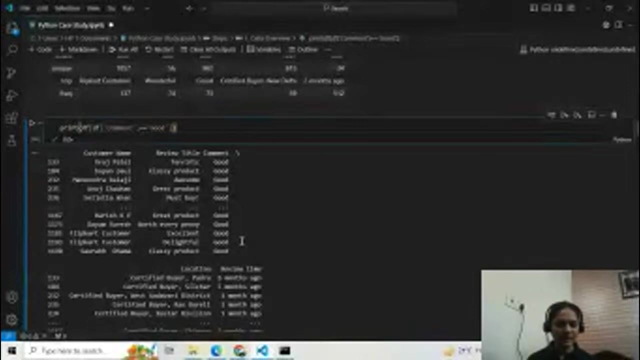 can see the view title until different and the common name are different, but still they have just put the comment as good and has happened over different time period where different locations. so, uh, there's no like correlation between time, lotion or you know name or anything the people have just put. 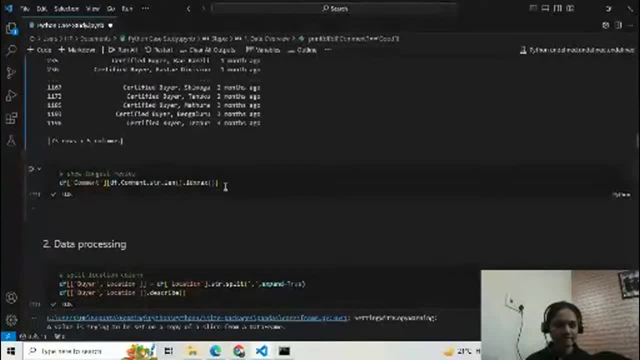 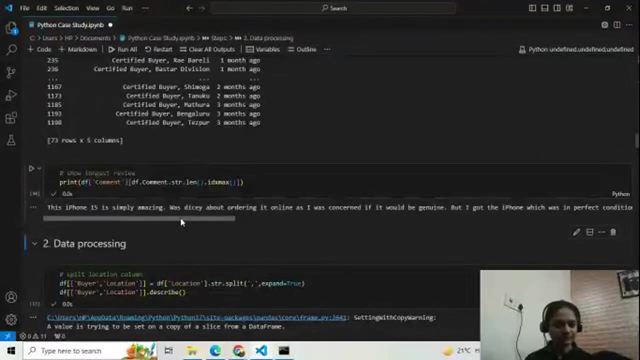 uh, good, as the comment, name comment and also you can see for. uh, let me print it. this is just you can of one word, reviews. you can see some people they take time and they uh thoroughly the product and put pretty long reviews. those long reviews are unuseful for you know the seller. 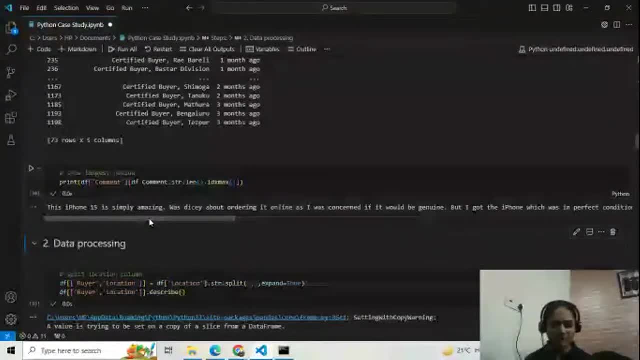 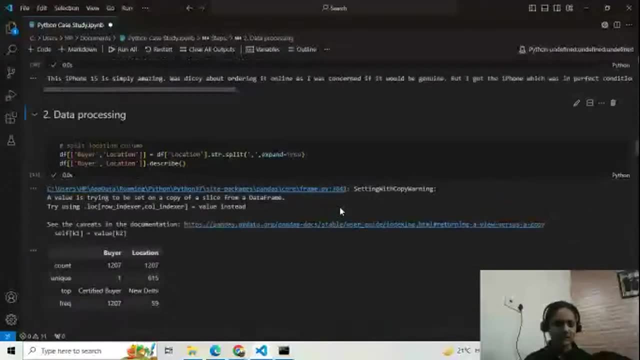 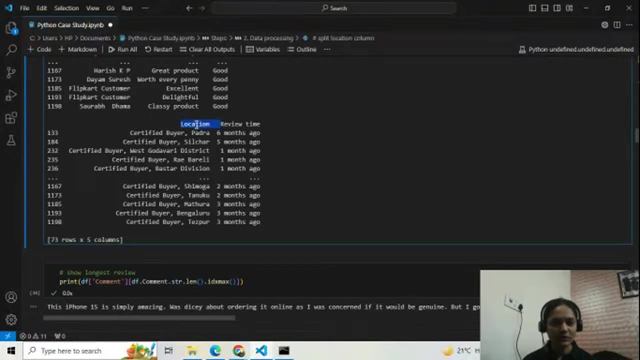 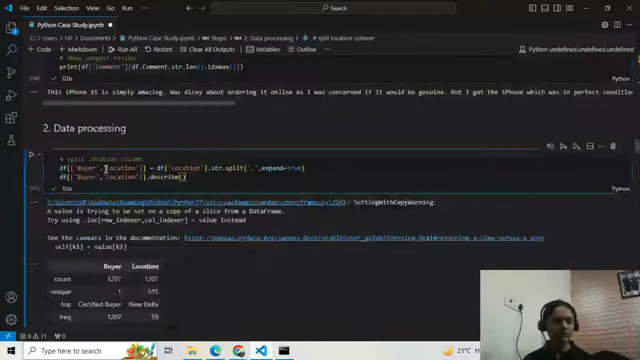 know more about like or what is they can put in the product. then we are going to move to data processing a little. so, uh like, as you can super a column, that location column, so this may actually tell you that there is a certain buyer, and then we have the actual location put here. what we have done is simple. 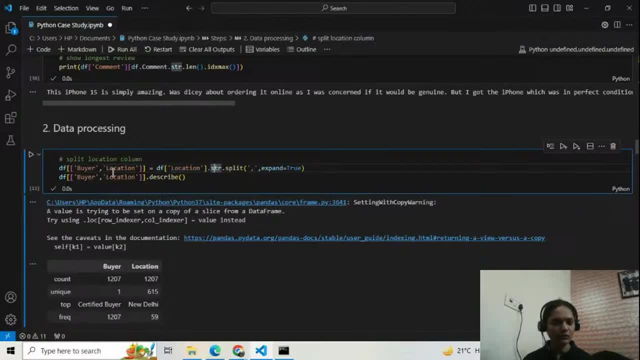 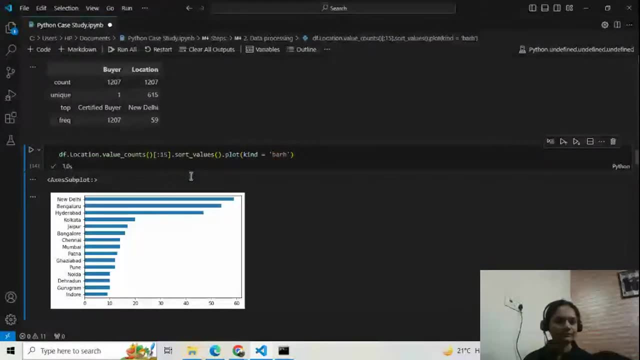 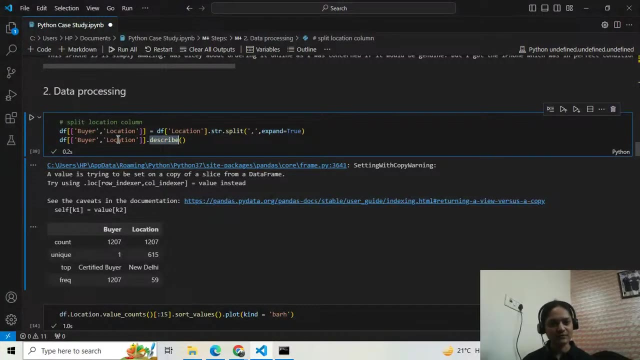 split your location. split into two status: the buyer and the actual location- right? so if we split this up, you can see we are again running the describe. so, as you can see here, we can run it over the entire data frame also. so as you can see same we have done. location- maybe checked earlier. there are around 600. 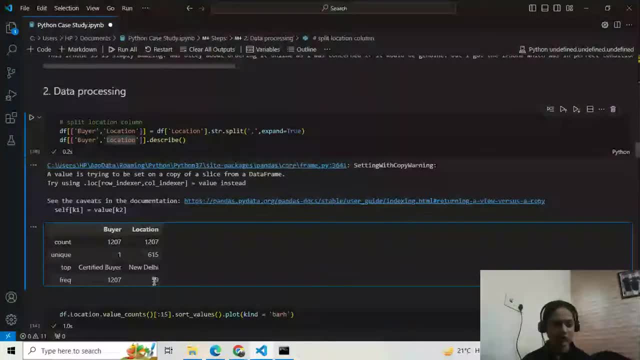 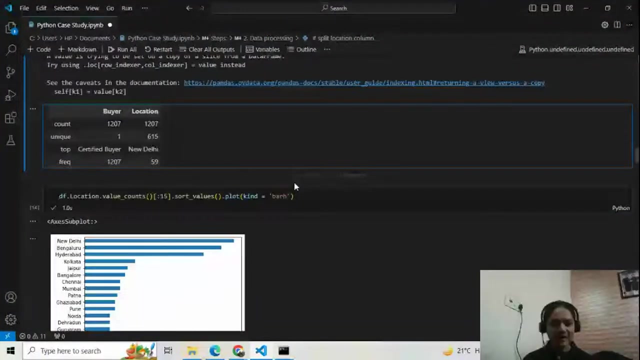 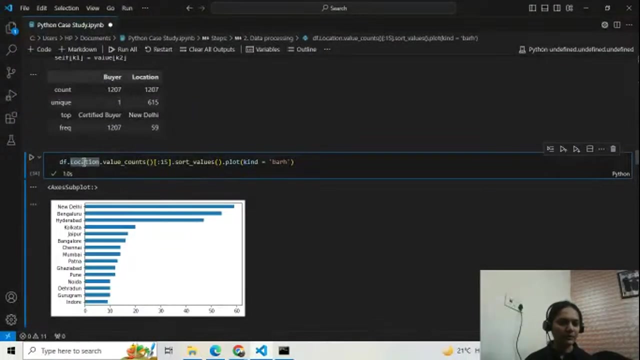 locations. just my new delhi is the top one with 59 uh frequency but. but as you can see, there's just one type here is fight by, otherwise you can see. everything has a name, so you can see here as a. we just sync top of the column from where we have provided the review. 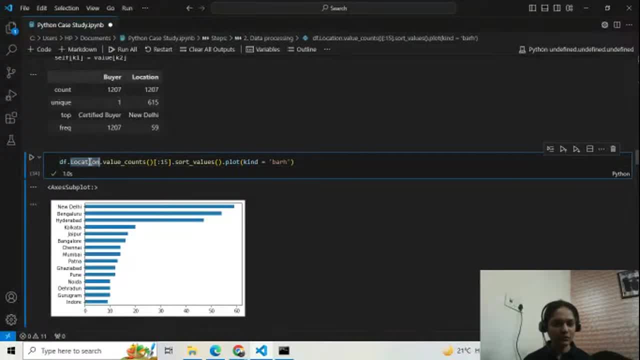 for that we have done value counts in the location columns of what pen is. value counts function is done. so when you have a column on which you are doing value counts, the unique number of values of that column. like you can say, New Delhi, Bangalore, unique values in that column. 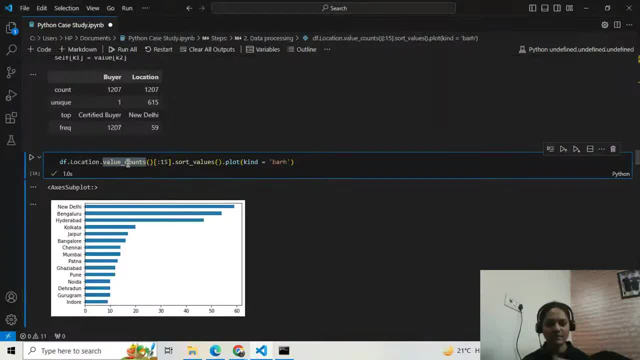 so function value counts counts the frequency of those unique values. so from that I took top 15 cities or areas and then I sorted them out. after that we are adding them so you can see here in this chart that this is the city in which the highest number of people have put their reviews. 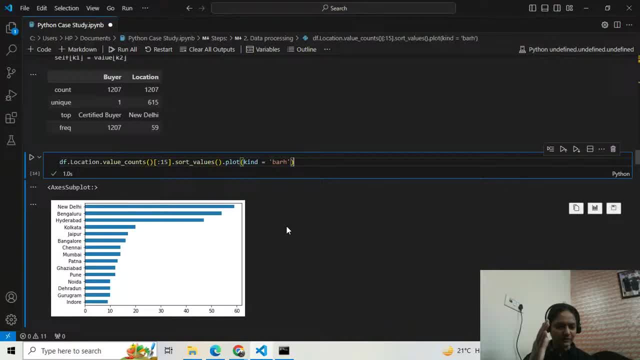 after that there is Bangalore, so we have these cities wherein people are putting in their reviews. so this could be interesting from logic guy point of view that where they have to open their warehouse, how to handle their logistics so that the most number of people who are ordering iPhone in places. 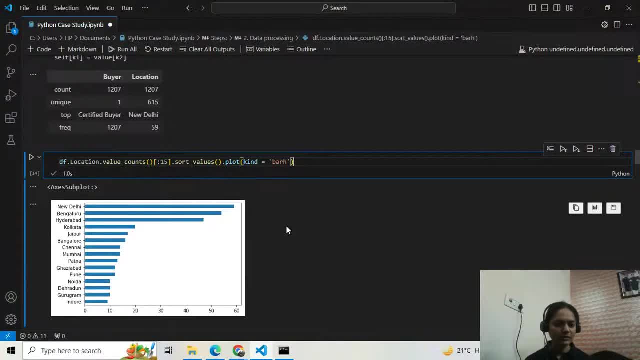 they get faster delivery or they have access to- you know- all the accessories to the iPhone and stuff. this is useful in that kind of scenario, but this is not a like. this will not give you complete, because, of course, this is totally only based on the review, not based on the interest of the people. 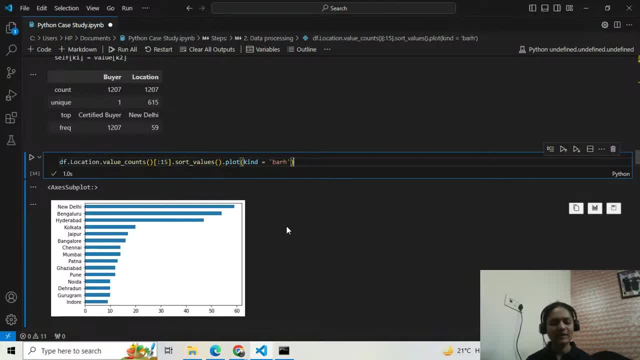 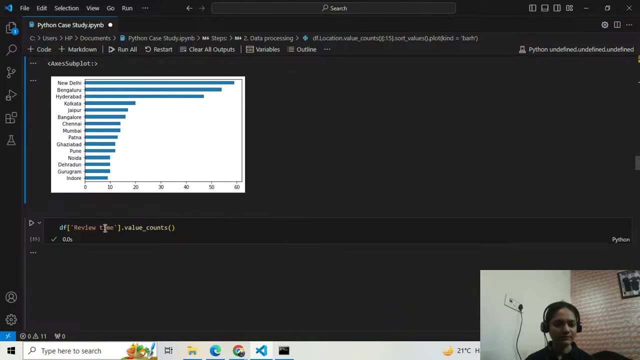 so we need to consider interest as well. so for that there are different ways to stack data, but for this study we are considering these reviews. basically, these are the top 15 cities where people have put the reviews of the product and same way we have, we can do value count for this also. 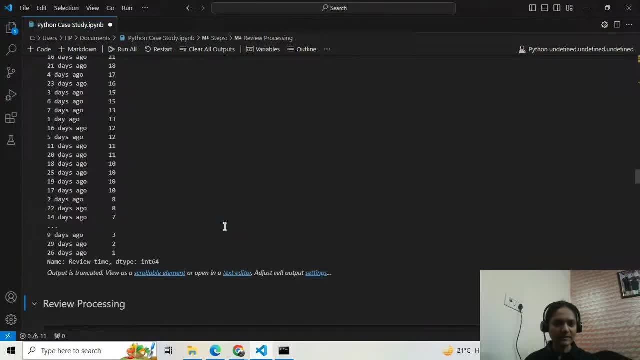 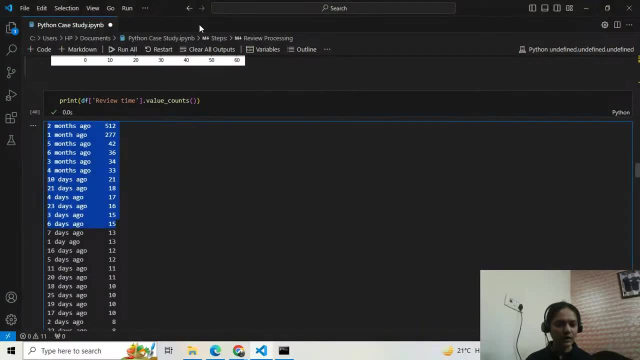 for review time. so review time, see this is basically since this data, like it was scraped today, so this date is relative to today's date, so like from today's date. 2 months ago maximum number of people put that review. so like we have, we are in. 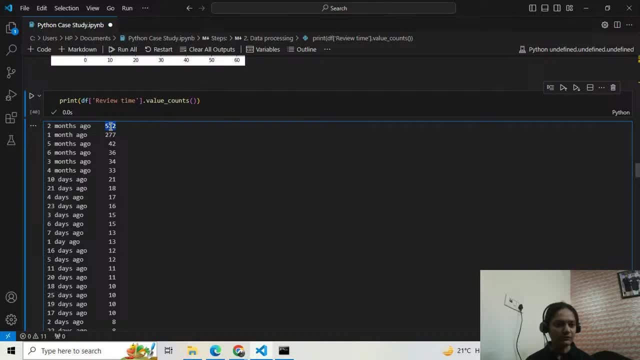 right now, so around in Feb, you can say that is when most number of people put their review. maybe they had this device for, say, few couple of, so couple of weeks after using it, they are finally getting the time to review the product. so there are different reasons. 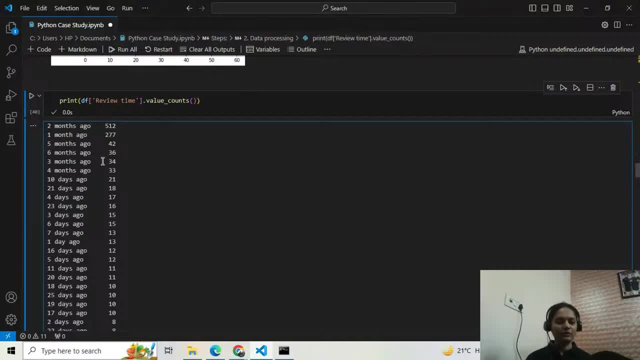 why specific month have the most number of reviews? maybe they had the product was on sale period. people purchased this product after one or two weeks. they are putting adding their reviews about it. so there are different ways but you can see the some time was 6 months ago. 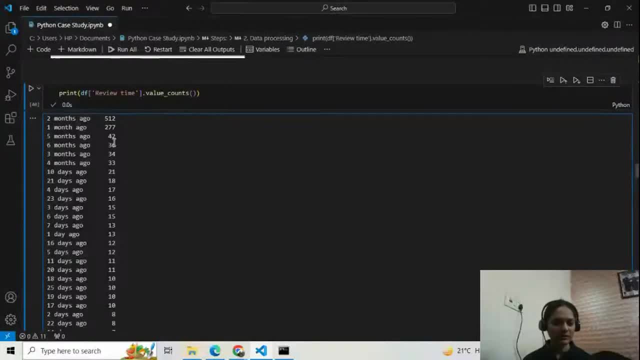 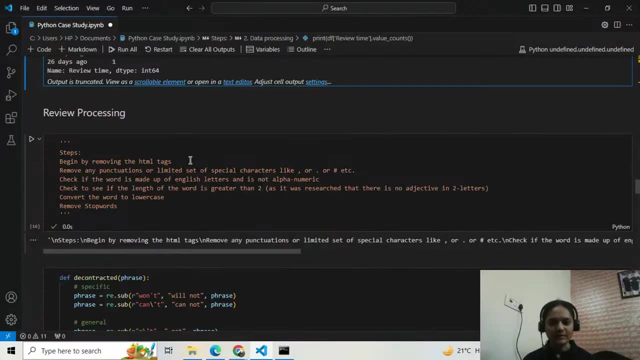 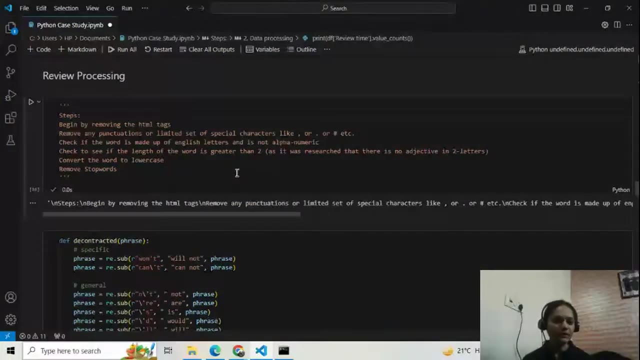 so that is when the product was listed on e-commerce- a little time before that, and that's when the review started coming for the product. okay, next we go to. so this was about little bit about the date. now we move on to the reviews process. so if we can do, 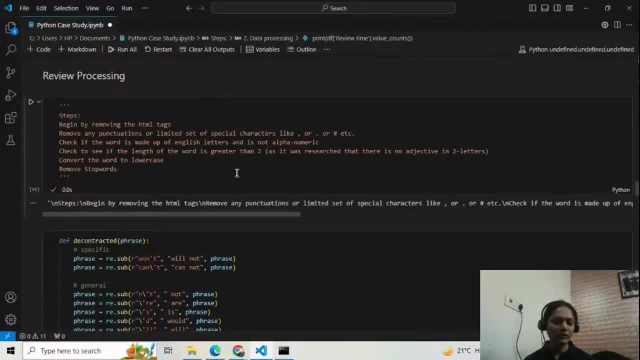 any sort of sentiment analysis data we need to process our reviews. first process. there can be a different steps, so I have listed out some common steps. there can be more or less of this step. this is not standard for it, so based upon your case use, you can add. 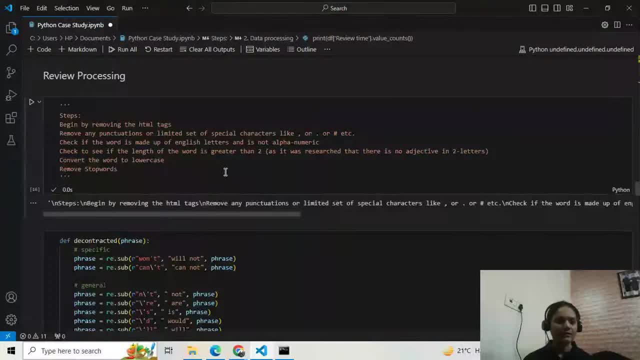 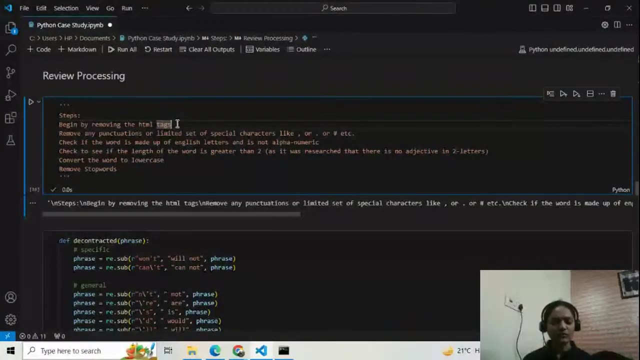 or decrease these steps so over. I am starting with like: firstly, we are removing some html tags. so often times we have and we have scraped whatever. so under that there there are some html tags like maybe you have seen it, like this bracket and then html, then bracket close. 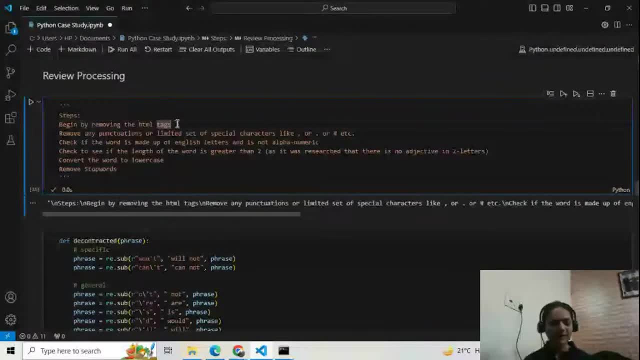 and then bracket close. that kind of data is scraped with comments, so we need to remove this data. also have some urls coming in, so those urls may not be useful in our final analysis. so that's why we are removing any type of html data from our reviews. 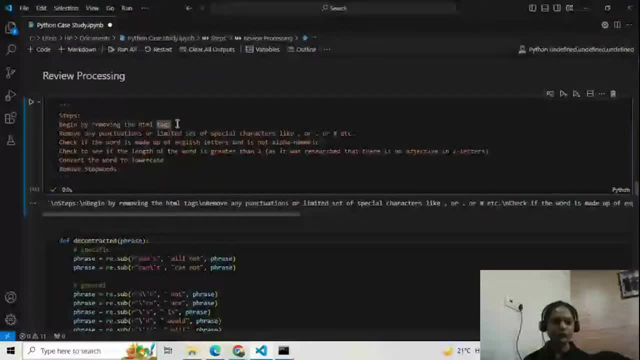 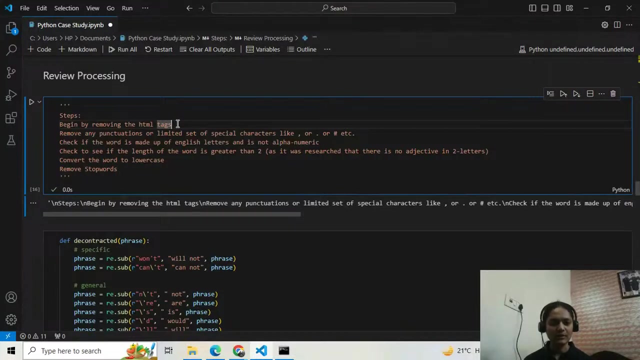 apart from that, we have some special characters. like we saw, there were some emojis coming in or there might be some hashtags coming in, especially if you are taking out twitter and facebook data. so there are hashtags, there are so many hashtags. and if you have instagram data, there are. 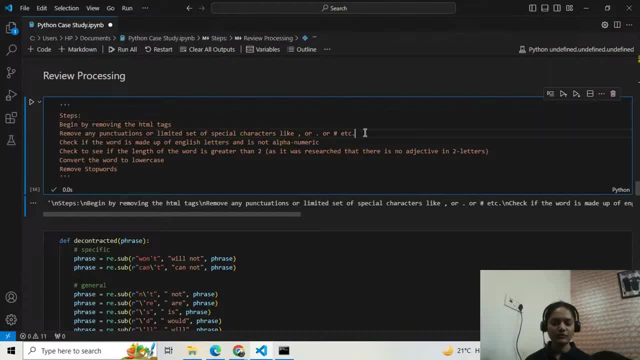 very hashtags or functions present, so we need to either remove any alphanumerical use from our data, so, since we are only considering english letter, so that's why we are going to be removing any non-english letter character present data, so that will be removed. 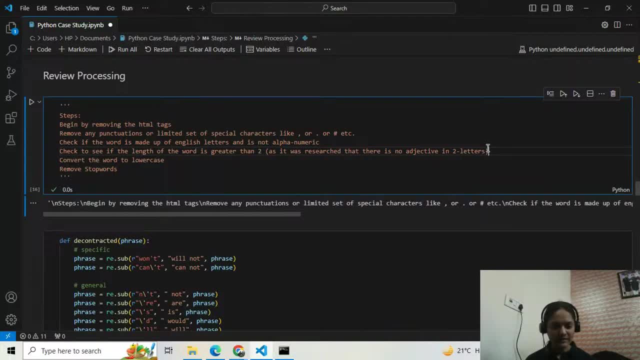 and next next step is for removing any small words. so if there is any word present in the data, so those words we are going to remove it. and final last two steps are: one is to convert everything to lower case so that we do not miss these types. 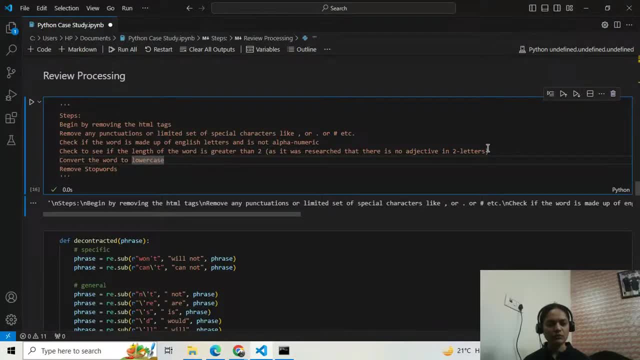 of petitions and finally, there is one step to remove these stop words. so what are stop words? stop words are words like pronouns. so stop words, words like pronouns, or you know, will not those kind of data present that do not add any meaning value to our 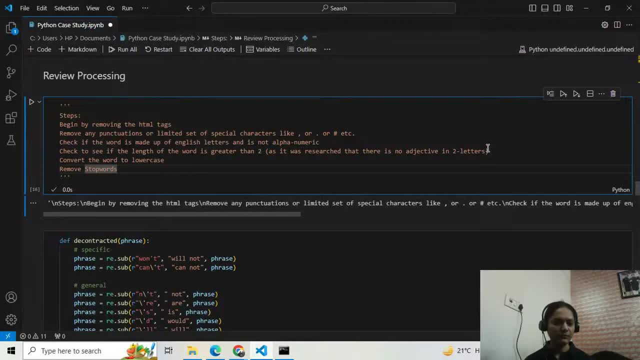 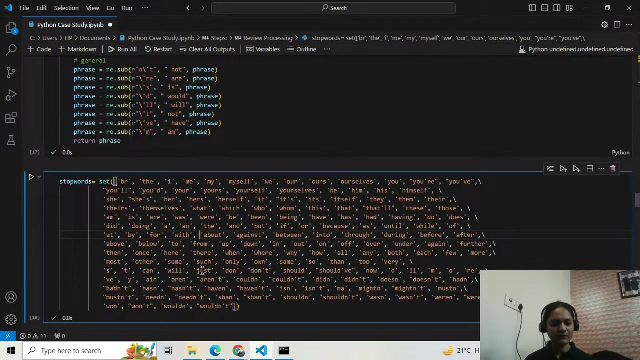 text data. so that's why we often remove this stop word from our text. so to remove stop words, there is in NLT library. there is a list of stop words in the list itself so you are able to see different types of stop words. so already available. 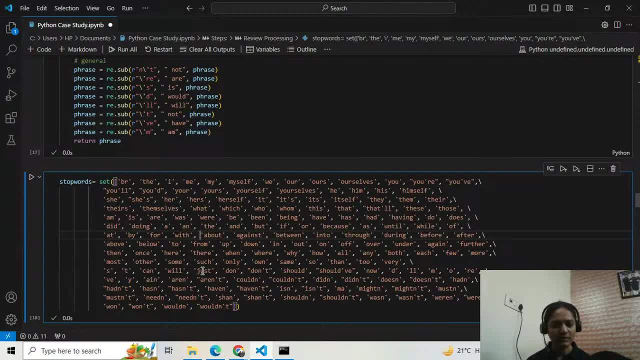 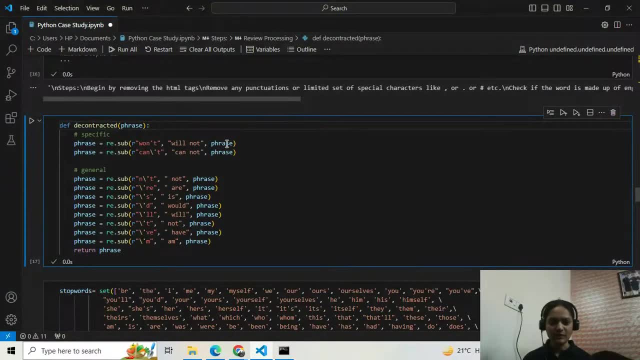 in NLT, but just show you that what kinds of stop words you can see in NLT library. so in NLT library there is a list of stop words in NLT library. so in NLT library there is a list of stop words in NLT. 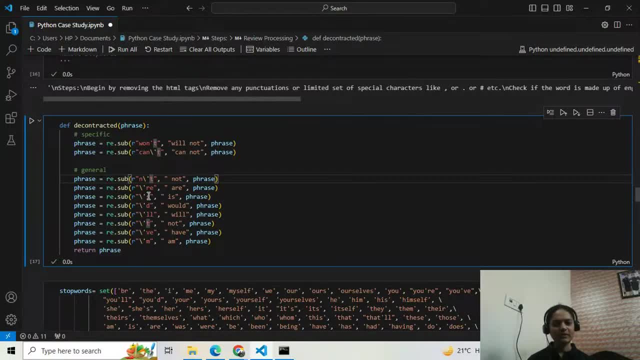 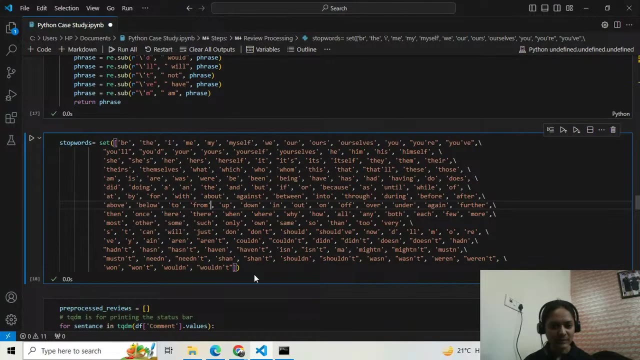 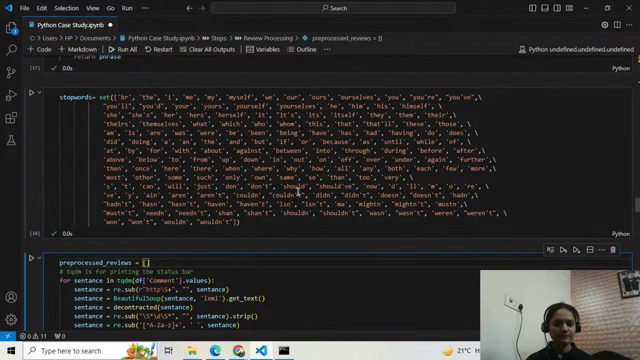 library. so in NLT library there is a list of stop words in NLT library. so in NLT library you can see the stop words in NLT library. so you can see the stop words in NLT library. so in NLT library you can see. 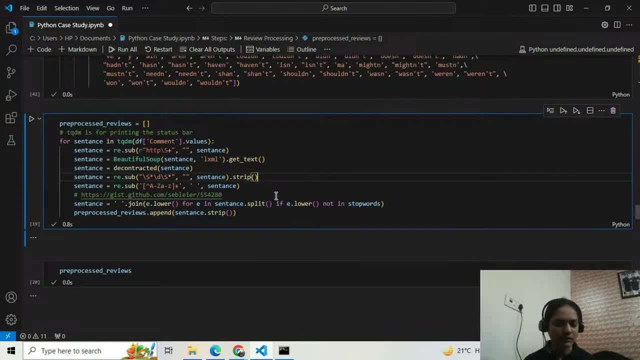 the stop words in NLT library, so you can see the stop words in NLT library. so in NLT library you can see the stop words in NLT library. so in NLT library you can see the stop words in NLT library, so you can. 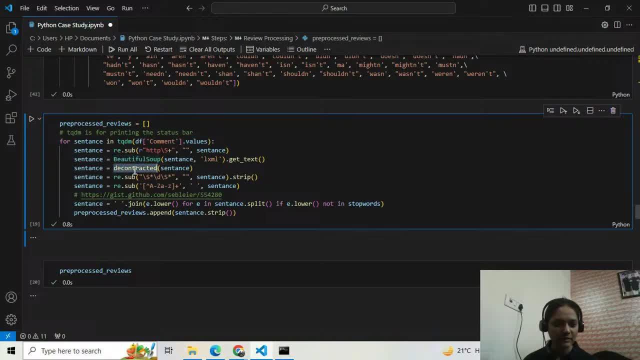 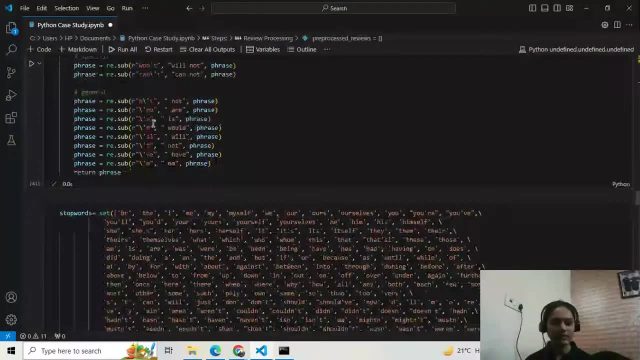 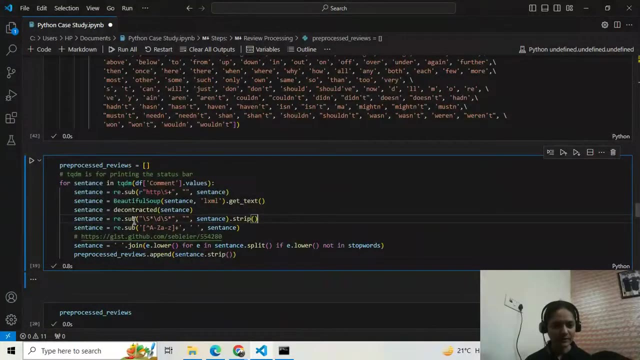 see the stop words in NLT library. so you can see the stop words in NLT library. so in NLT library you can see the stop words in NLT library. so you can see the stop words in NLT library. so you can see the stop. 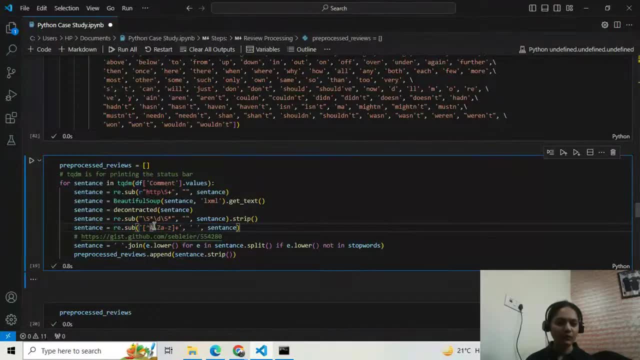 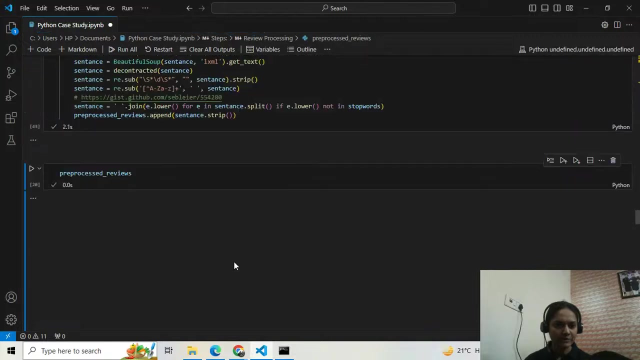 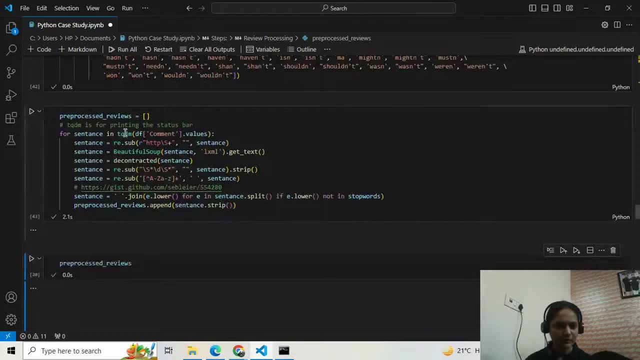 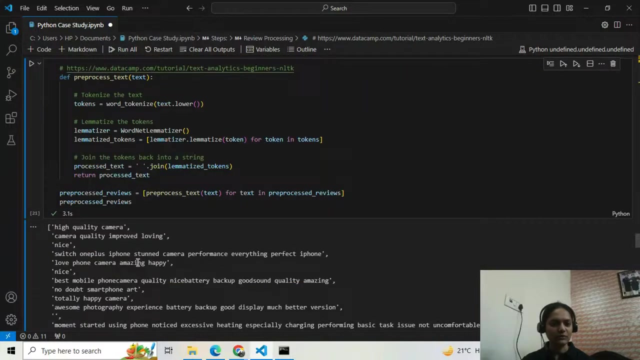 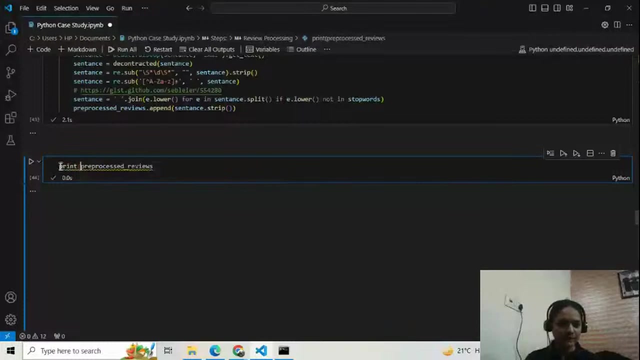 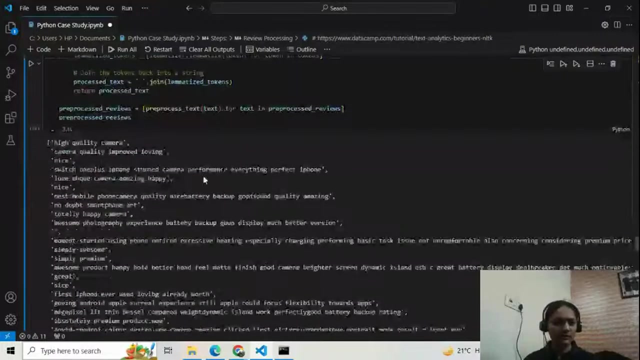 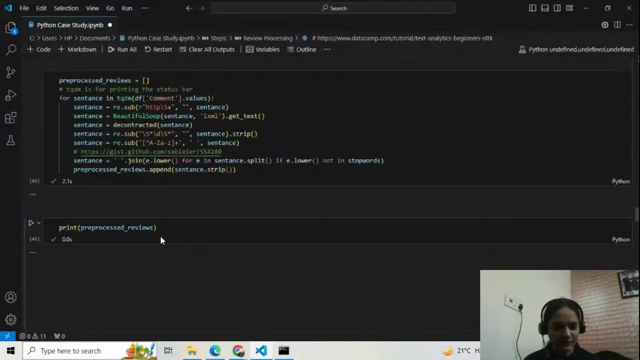 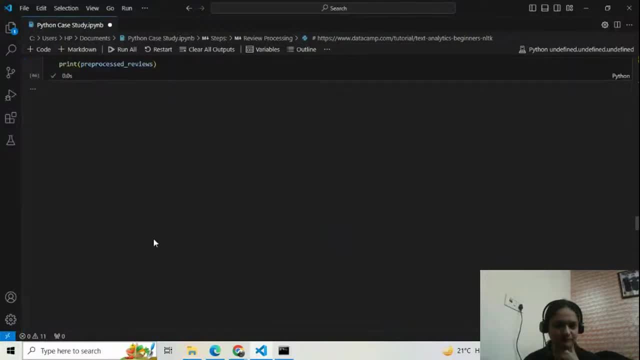 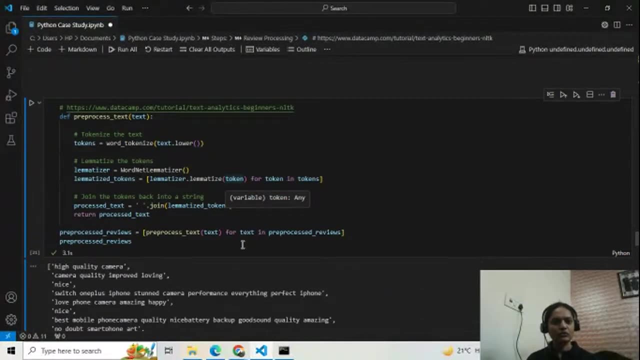 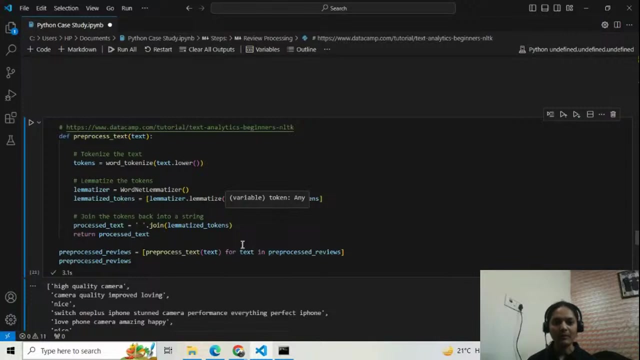 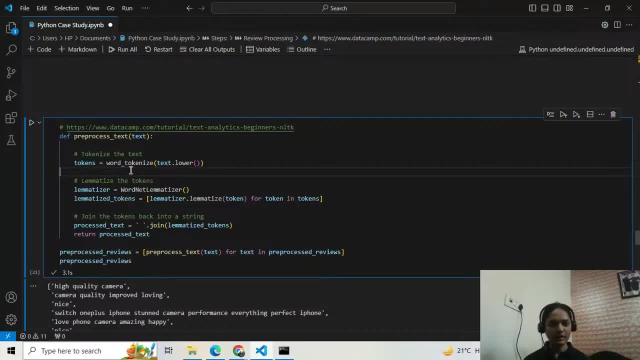 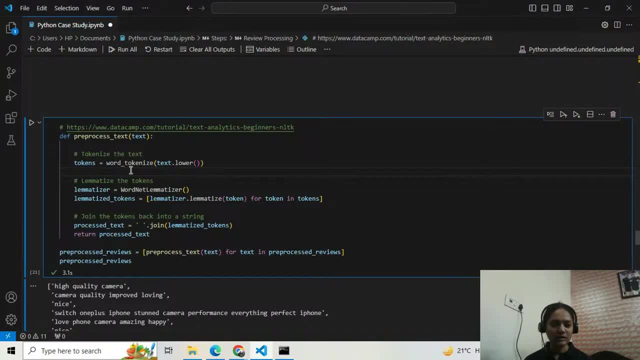 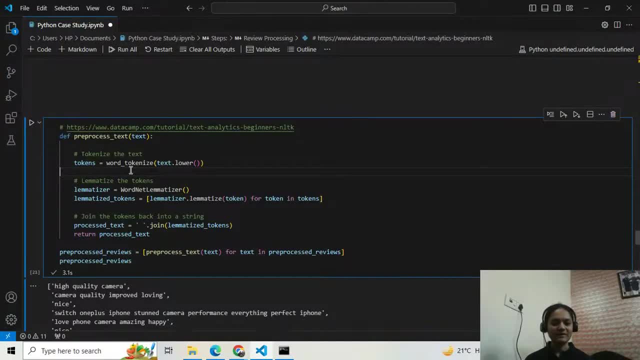 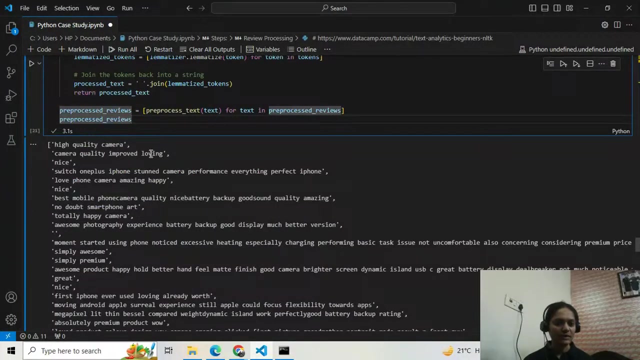 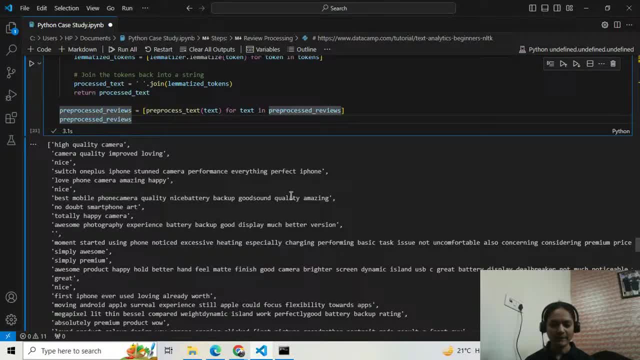 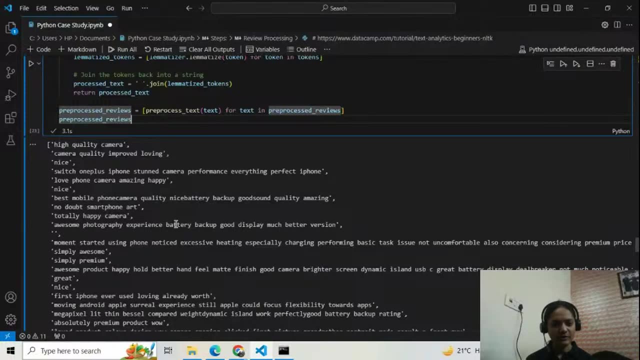 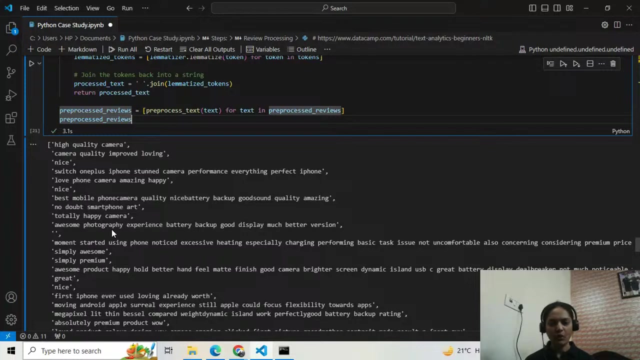 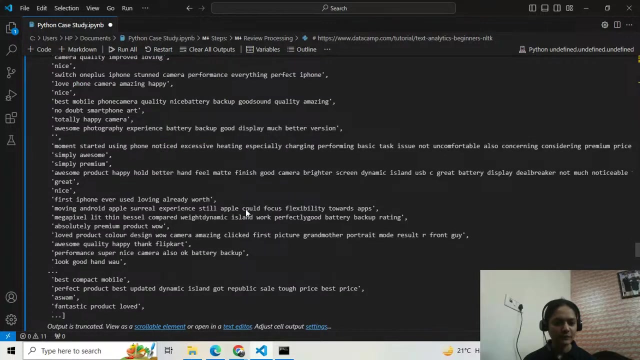 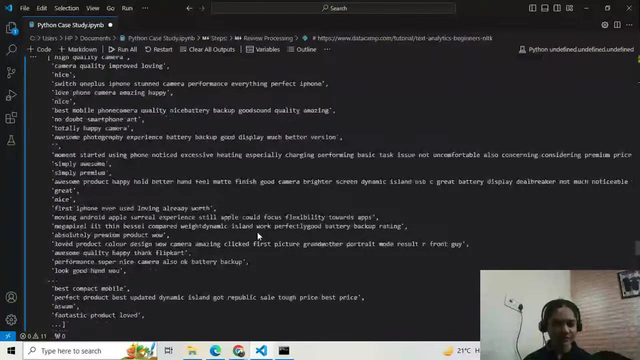 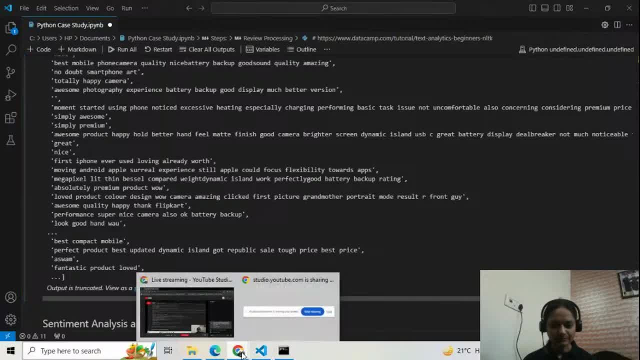 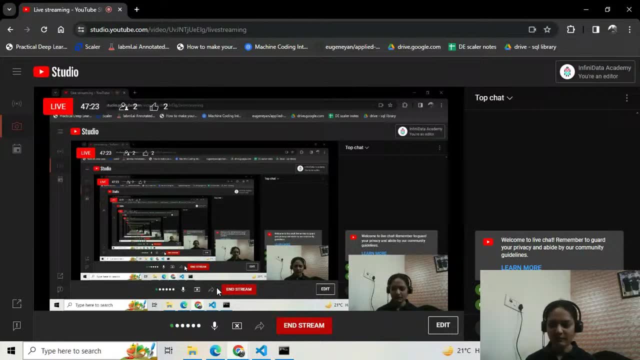 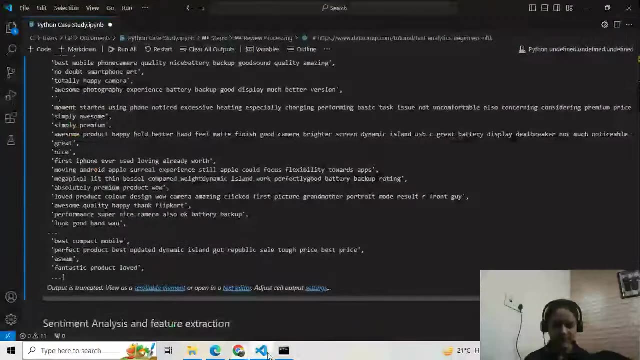 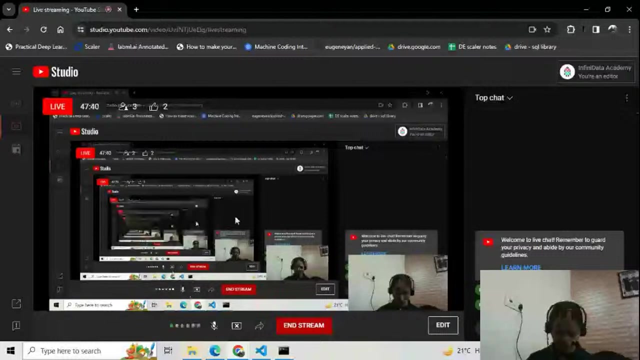 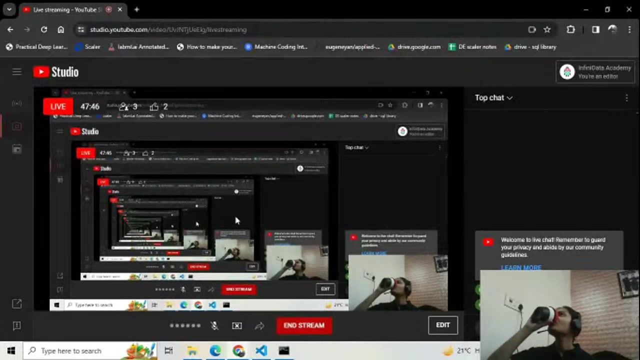 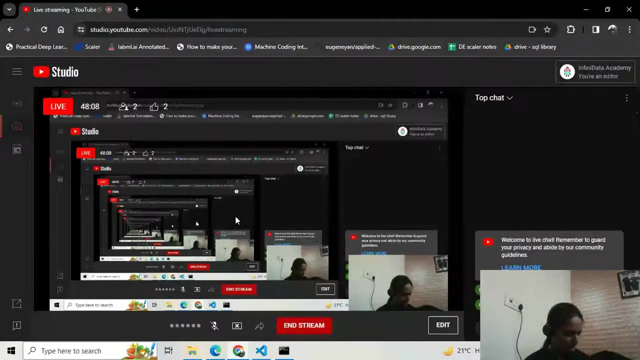 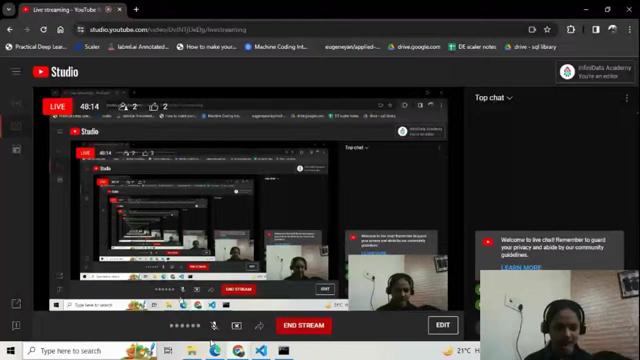 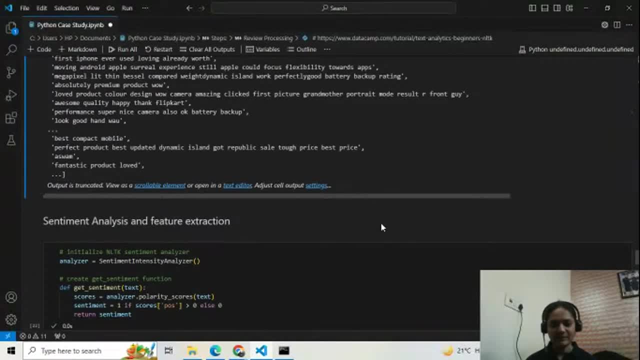 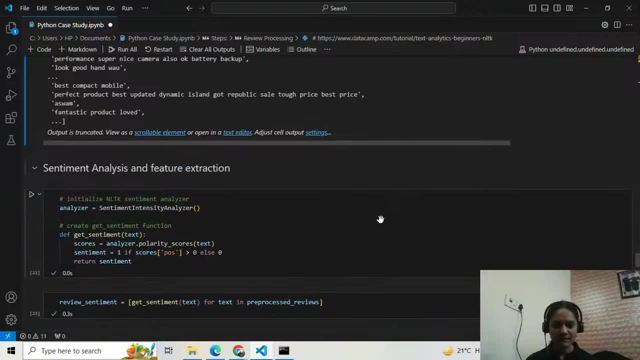 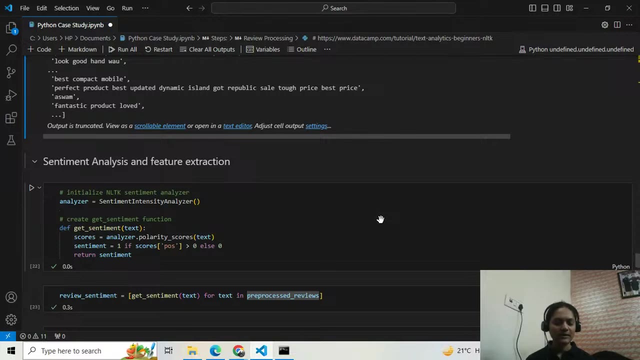 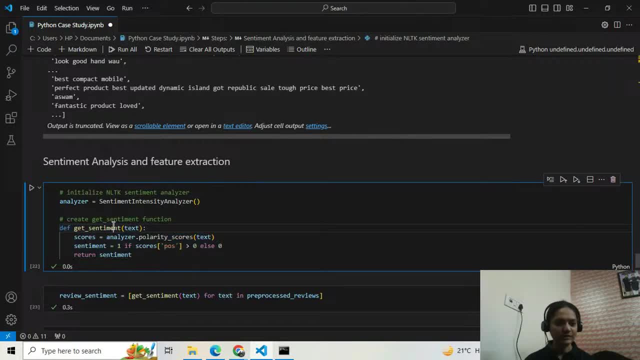 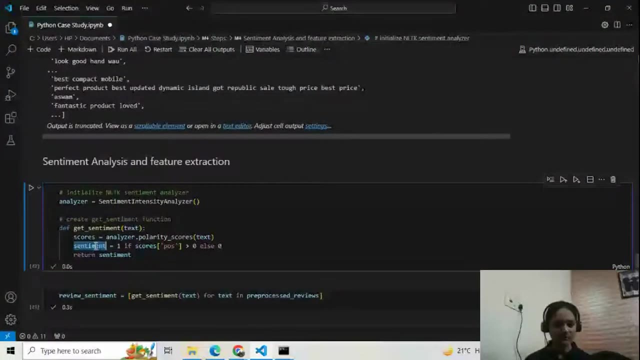 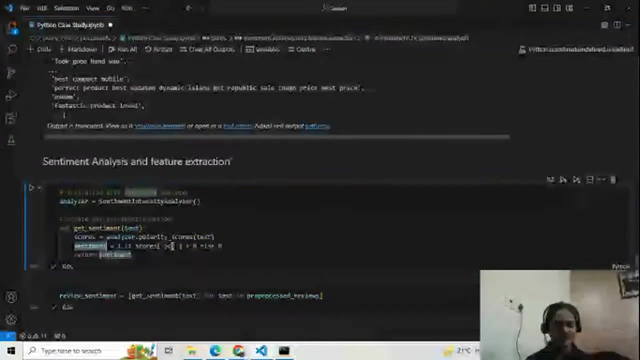 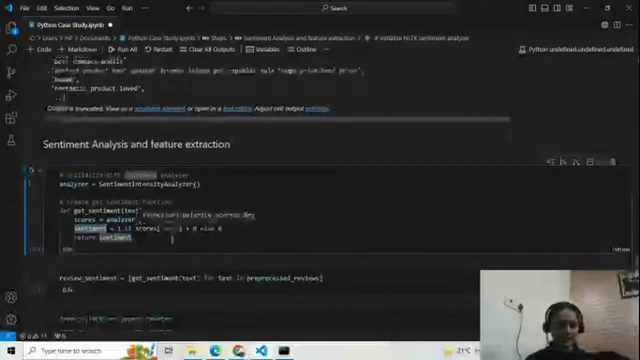 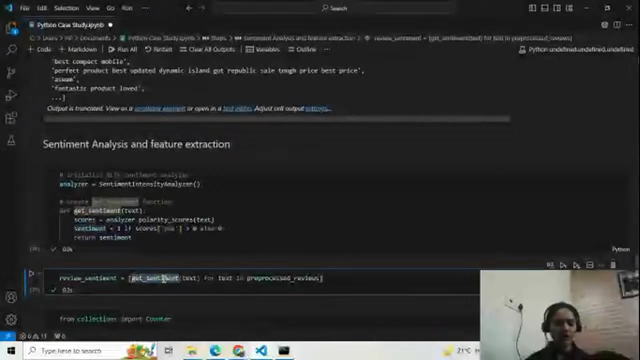 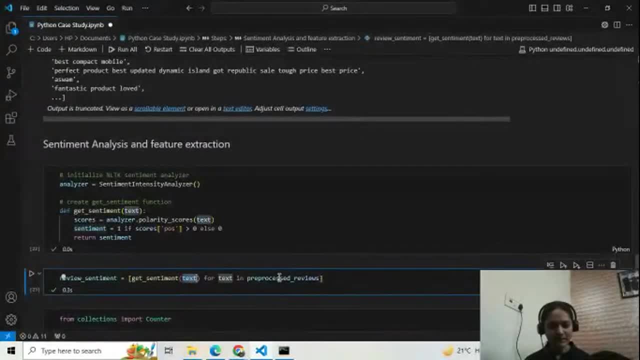 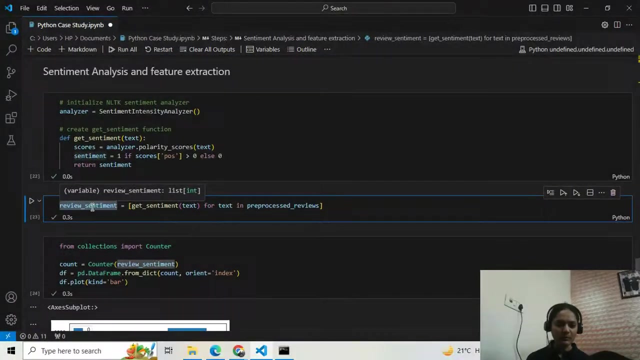 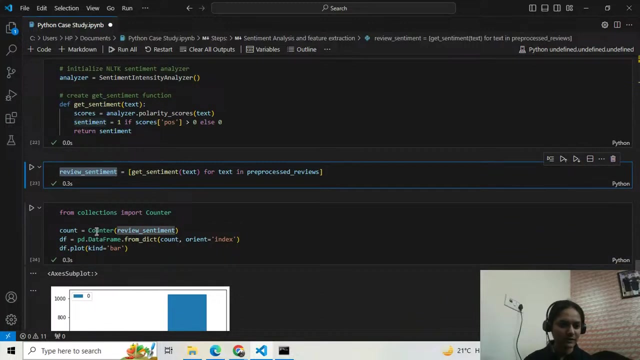 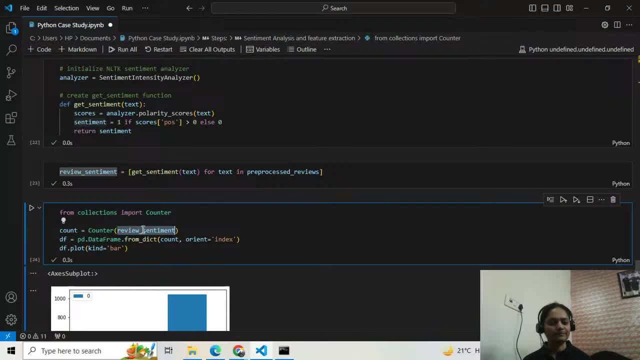 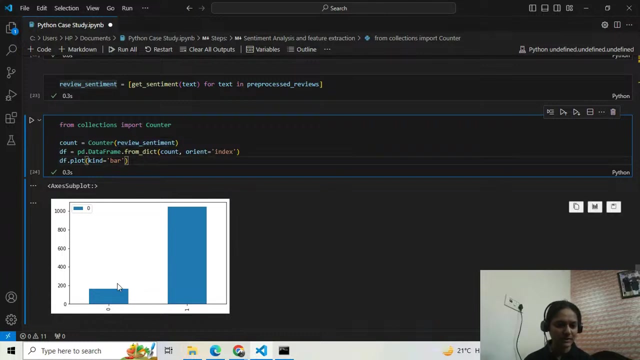 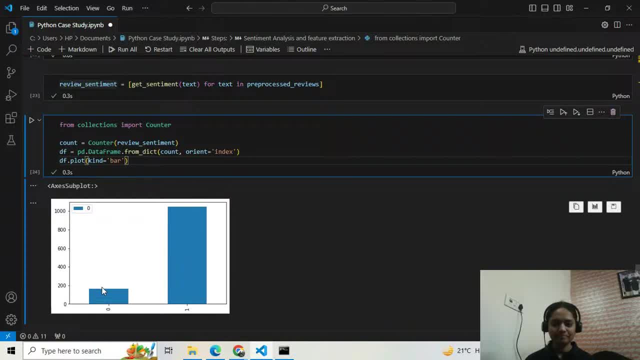 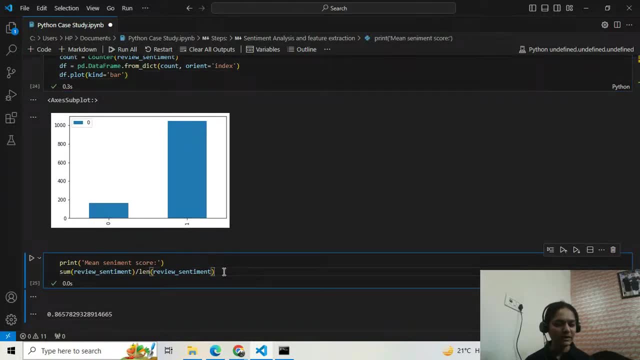 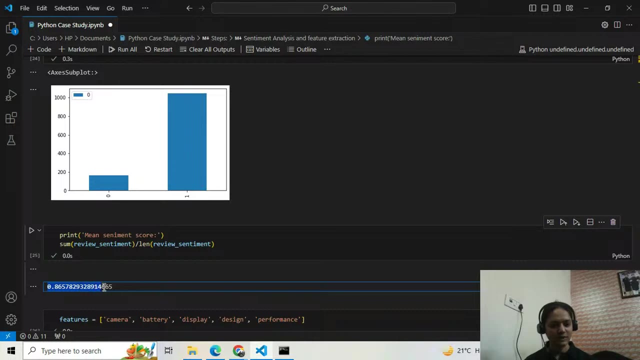 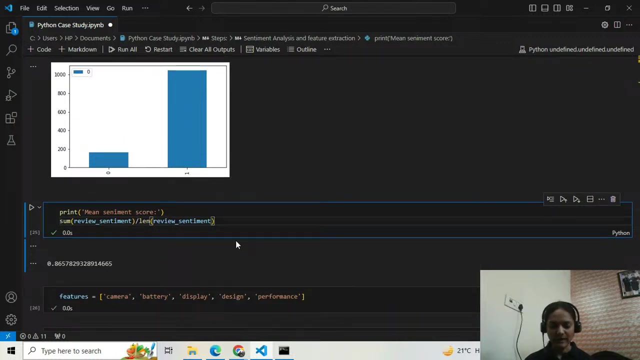 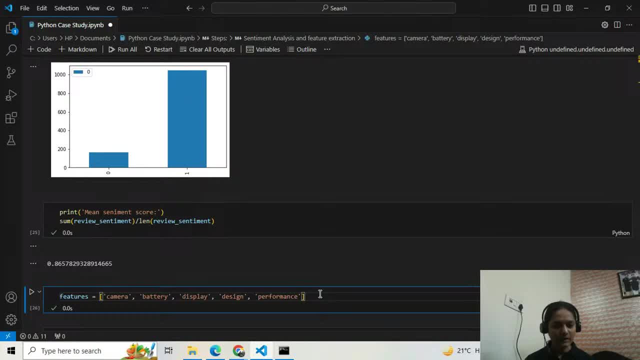 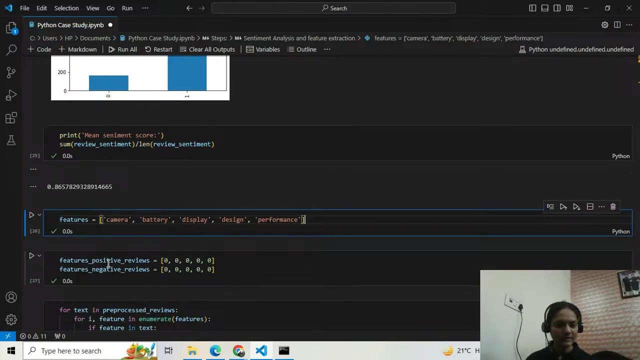 can see the stop words in NLT library. so you can see the stop words in NLT library. so you can see the stop words in NLT library. so you can see the product. you know, Nick camera Mentioned here and and those reviews are positive and negative. review starting the camera. 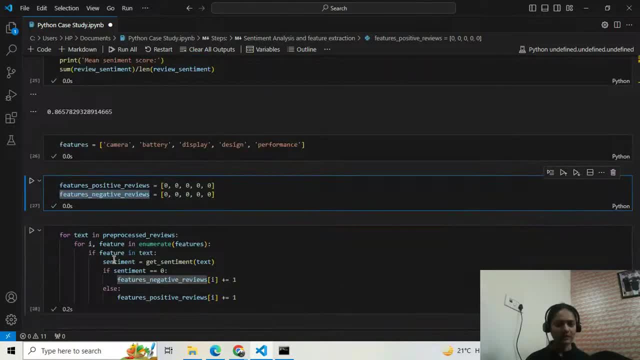 Right, So is Kelly a. basically run this for loop, for loop, may. we are taking all the process review and Uska and we are checking for each field feature. We'll particle text. my president taken a. that is a user name camera up: Nick Toby comment. 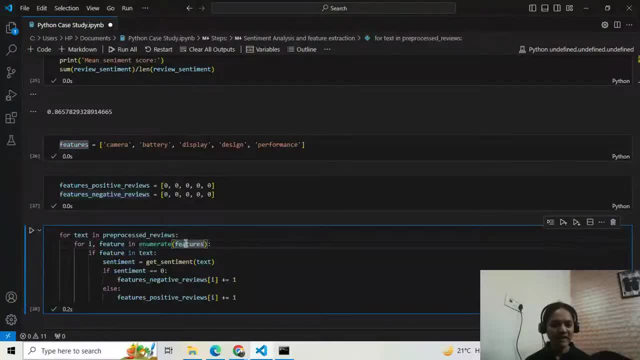 Us map mentioned here. Yeah nahi, Let's say comment: kill a camera quality very good. So whoa as a camera, Whoa as a lick, whoa, If I huga just make a camera feature available. Feature feature is just a like table over here You can see: use, make camera, but available has. so that is identified. 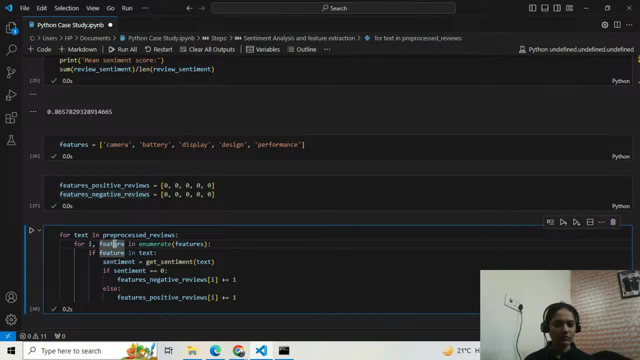 in my, In this or who's may be a, just taking a sentiment key, I got camera, My particular table, a bullet, Oh it's got sentiment. Yeah, I again using the same function as upon job, a functions get Function. that sentiment was co-user getting a treatment. and then we are checking a girl was sentiment negative. 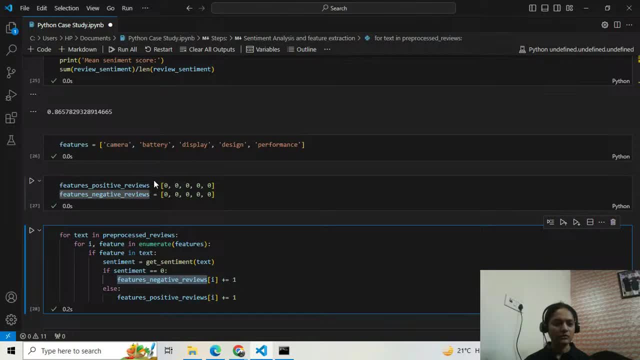 Hey, I'm a negative guy But are a, so basically my review may. cameras are related. I don't think negative is mentioned. So whoa Joe, negative review here. camp position camera is at the first zero index. So 0th index page, a guy and it will increase the counter to. but 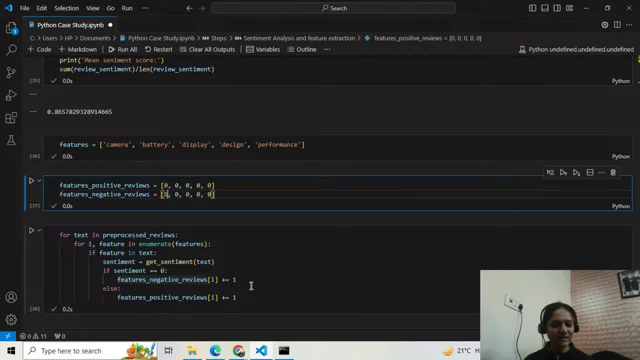 Right, and let's say, if you camera said related- and those may be, that is the review is negative. It will, you know, increase the value from 0 to sorry. what to do? so, as a, Have a final List, just made them reviews home. get, just make cameras, have, just make a mission, and that will review negative. 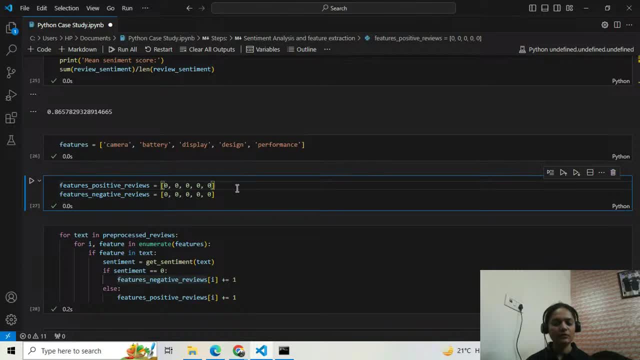 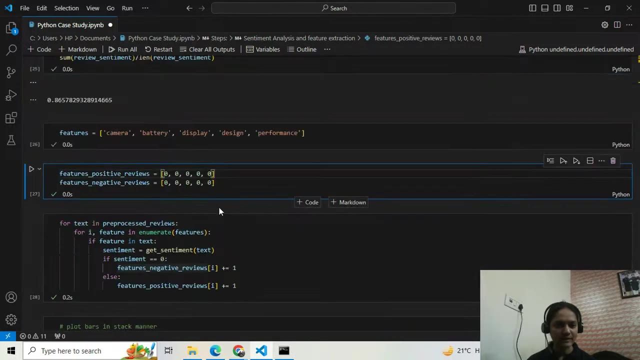 It's a final features: positive risk make yoga will have number of reviews. count of number reviews: Just make camera out. these features are mentioned. They are negative in nature, So it's called execute. Finally, It's called a date. Yeah, and this data frame was. 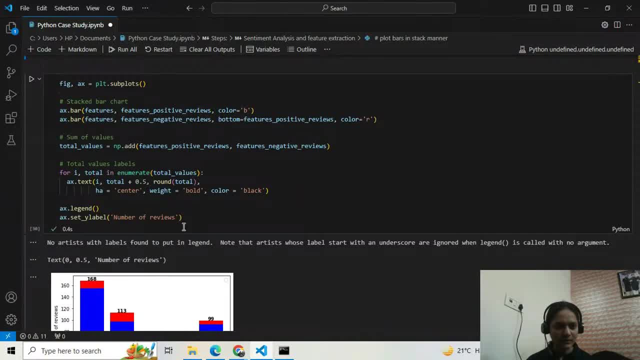 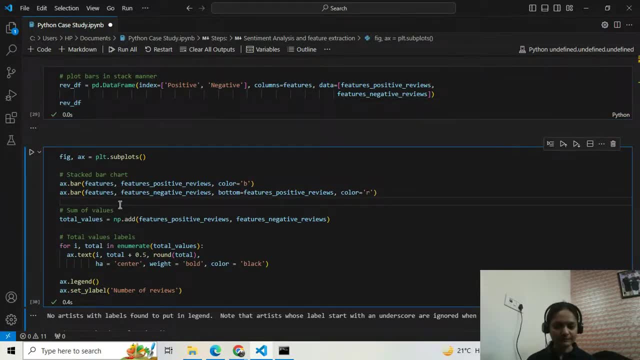 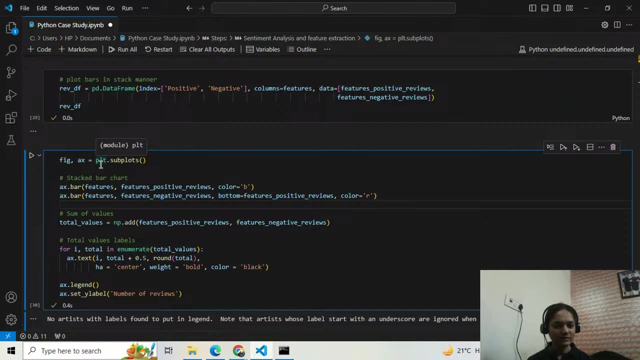 being shown over here. all right, it's my output in Europe, but we can look at the visualized output over here. so Position me. you can see. this is the code, may? we are just Visualizing this. data, that is for each feature We visualize, is count of positive and negative reviews. 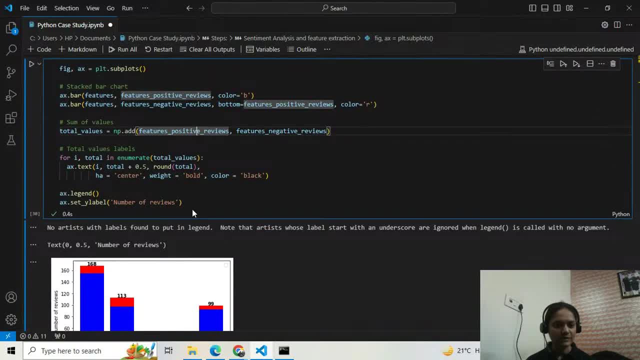 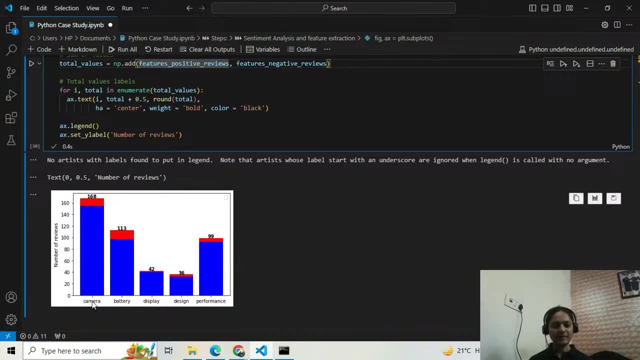 right and skip. just Seeing kick it mean a total number of river, So you can see a total reviews. just remember a mention: it that is 138 and all that with majority positive. around 155 is positive and 13 are negative. same for no other features. for other features you can see and so you have a design perspective, say this: 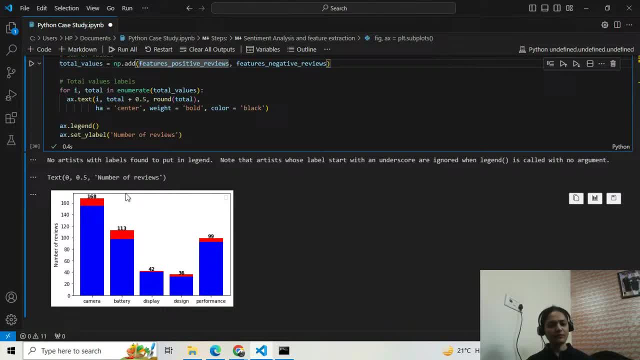 Set could be useful. key member of negative Related to battery people are: maybe they are very happy with the display But they are not happy with the battery. or they are happy with the performance, you say, but they are not happy with camera quality. So this kind of in you can generate from this date or a scale of a we do further analysis over for the like. 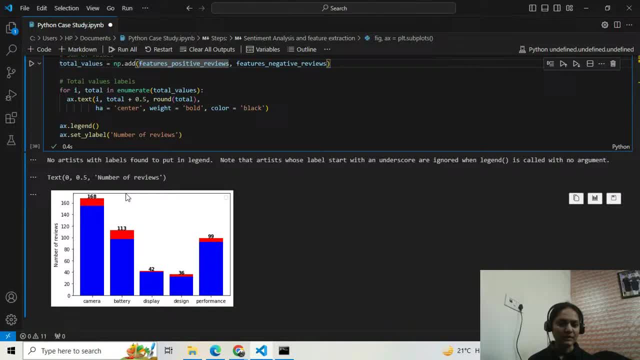 marketing case scenario. key cons area: may There is very less penetration but we have a as per the trend There's like a very high it worth individual. I do about it. So for my point of view We can have that kind of. We can have that kind of case study also different implement K according. we can have different get study. 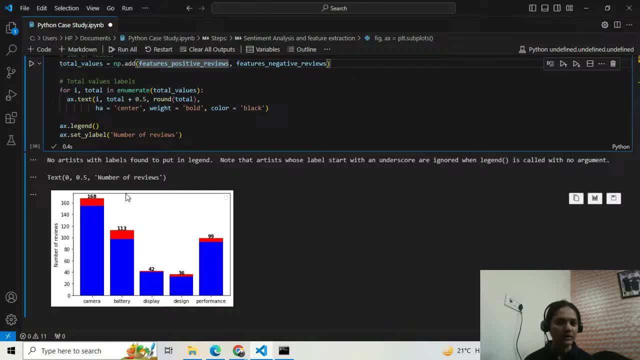 Basically we mentioned we can have the warehousing capacity Kind of case study and this one could be on the you know person building the product design. so unco reviews caring they can take a key. okay, they need to walk on the battery now they need to. 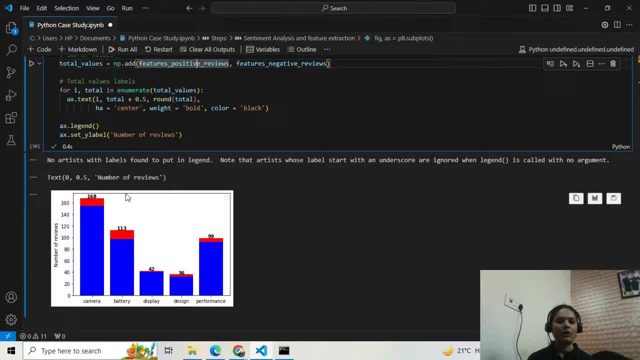 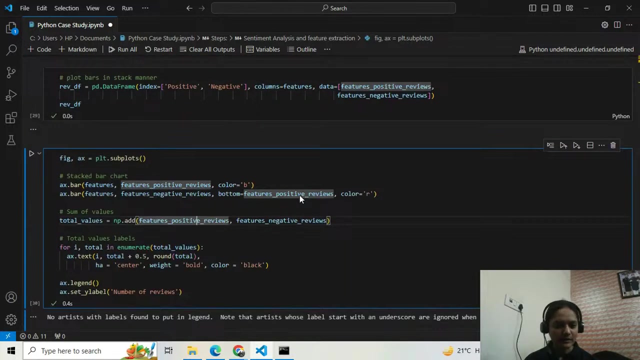 display of comments next. so so, as per the different types of uh insights that you know department or that are you know working on this product, they are, they can uh take. uh, they can take the final action based upon right. so this was the thing that we i wanted to discuss. uh related to: 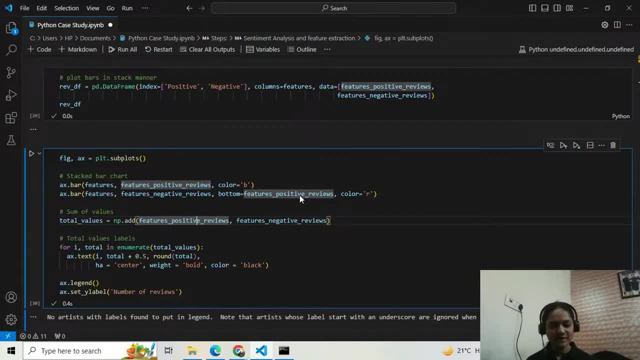 our case study. so this is very basic case study. there are, like in real world, case scenarios. there are like a very advanced analysis that people that we do on the daily basis for our product. so if you want to learn more about kind of uh, real world case study, please have catch, get touch in with our team. and although we have our data, 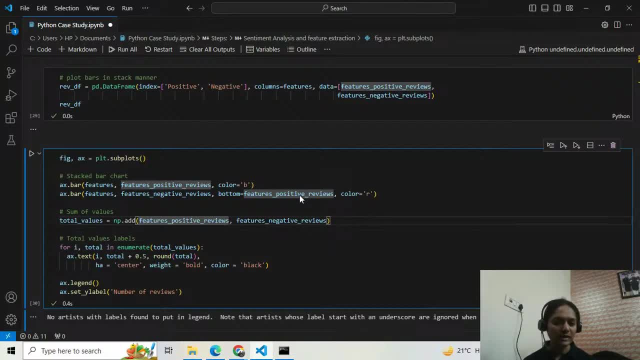 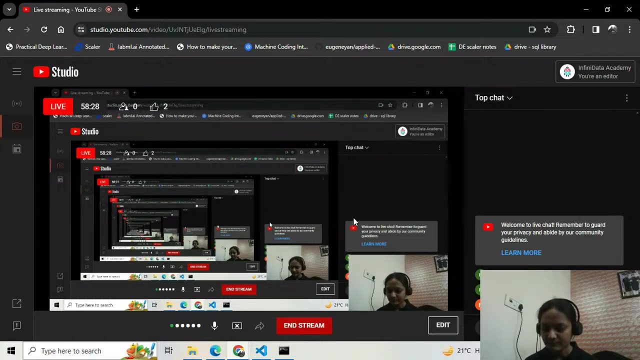 science starting soon and if you know details about can follow us on our linkedin and visit our website for any color counseling, so you can get in touch with our team. we will be very happy to with you guys. and so that was it about it. that was it about it. but if you guys have any question, anything i've you can uh. you can uh put it in the 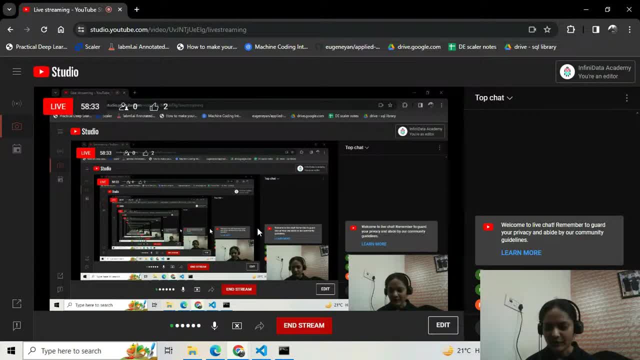 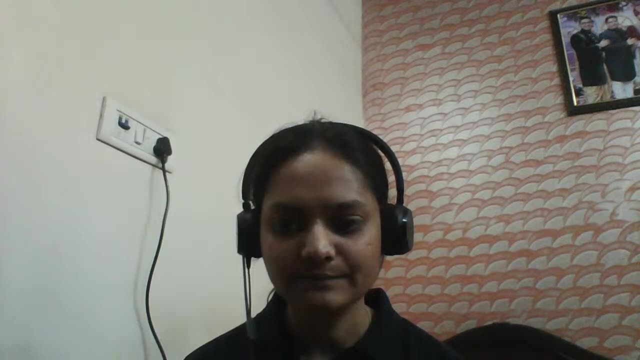 live chat. yes, navindu, if you have any question or doubts or queries, please, uh, add it in the chat and we can discuss this over here of. or if there is anything you want me to repeat, uh, we will. we can, you know, discuss that. so, navindu, if you are there, please add your queries over there. or if you just want to say hi, so,